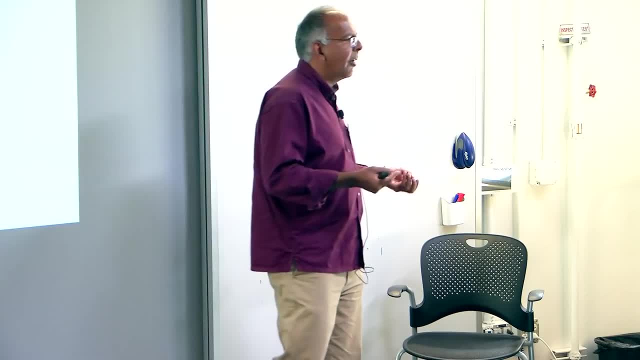 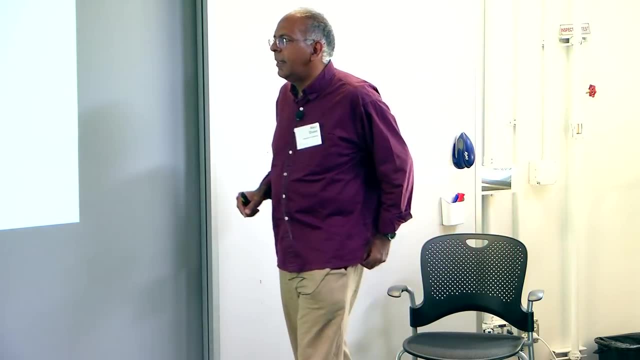 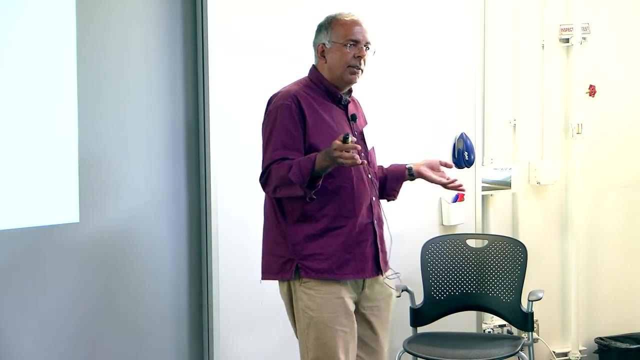 I want to pick up certain methods that are commonly used in the field of finite and algorithmic model theory and illustrate those methods by means of certain illustrative results. That's the general pattern. Now I realize that there are some people in this audience. 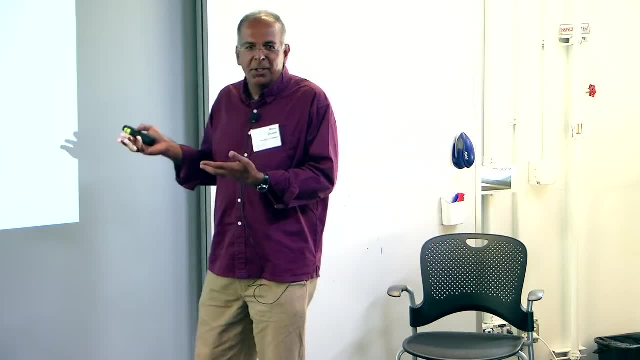 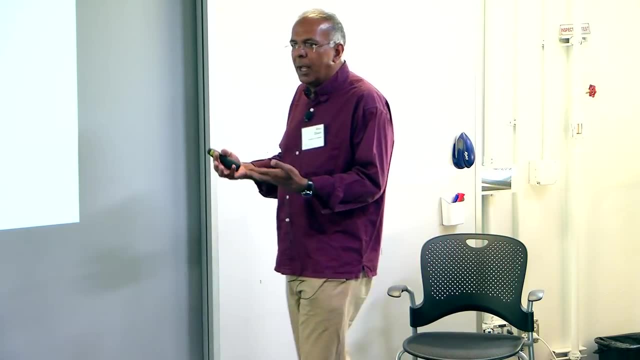 who know more about the subject than I do. There are others who know perhaps very little about the subject of finite model theory, So it's addressing this diverse audience. I I mean I hope I mean there's some of you who will find nothing that you don't already know in. 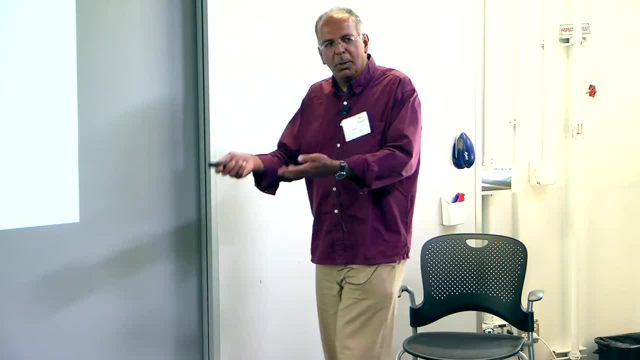 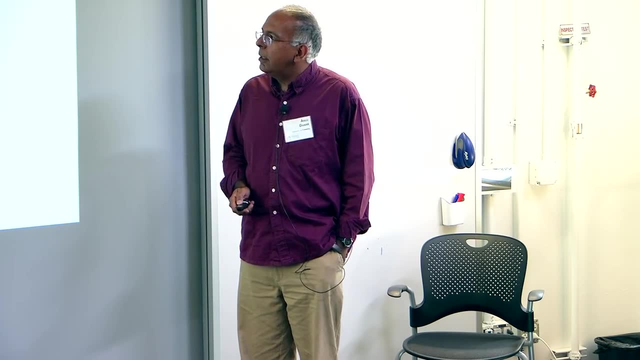 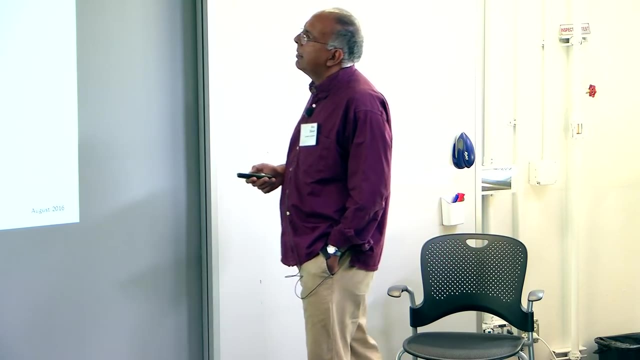 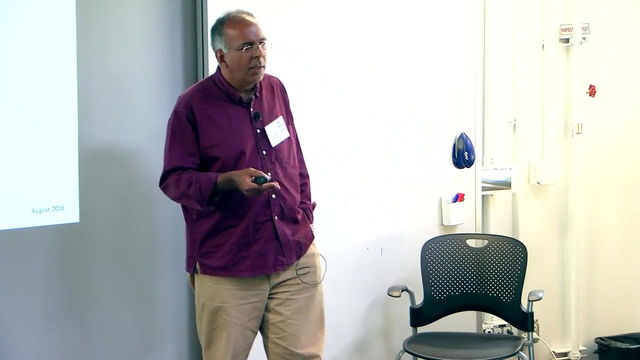 the first couple of lectures, but I hope you know you'll find something of interest as things go on. So, without those preliminaries, what is this all about? As I said, I want to focus on methods And essentially I think the term finite model theory emerged in about the 1980s. 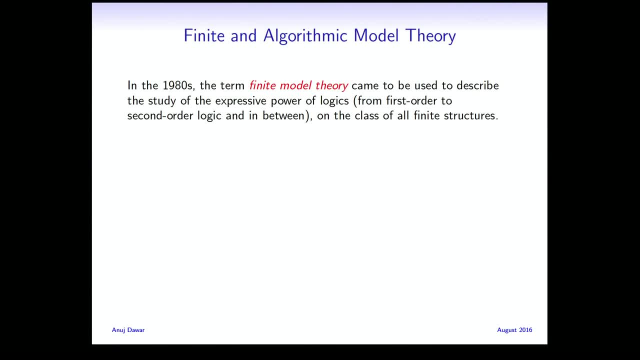 I'll defer to Fokion who I mean. I asked Fokion sometime last year and I asked a few other people who first used the term finite model theory to describe this subject, but nobody seems to remember. Anyway, it came to be used as a term to describe the study of the expressive power of logic. 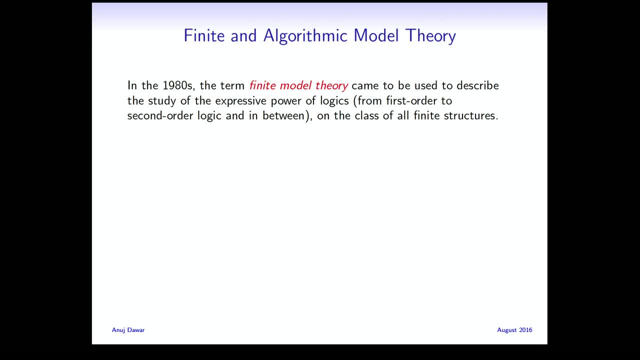 things like first-order logic, second-order logic, things in between, In the context of finite structures, the analogy being with the study of model theory, which has typically been concerned with issues of definability and expressive power, in the context of infinite structures. 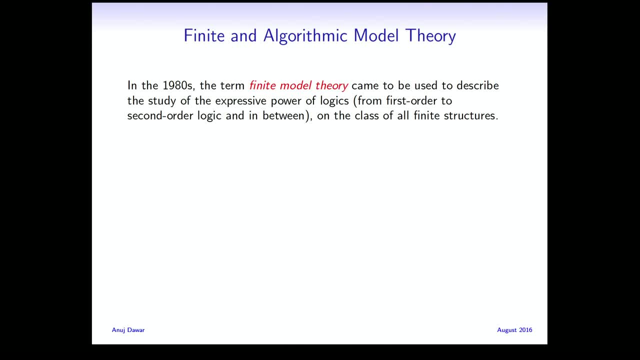 The analogy is loose because the methods turned out to be very different, and I mean the relationship with model theory as classically understood is sort of a bit tenuous at best. The motivation for studying finite model theory came from computer science, right. 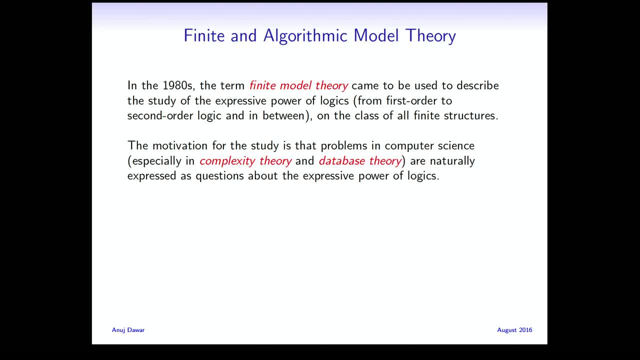 I suppose, especially initially- database theory and complexity theory, And the motivation is essentially that many questions which arise in the context of complexity theory and database theory can naturally be expressed as questions or understood as questions about the expressive power of certain logics and hence the need, if you will, for developing 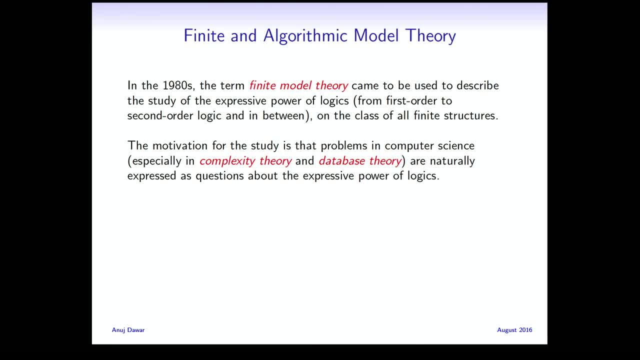 tools for analyzing expressive power. Now, essentially, I've said finite model theory. The title is finite and algorithmic model theory, Proviso here. When we talk about the expressive power of logics, the ones, the kinds of questions that arise in these fields, at least initially, as I said, back in the 1980s, people said: 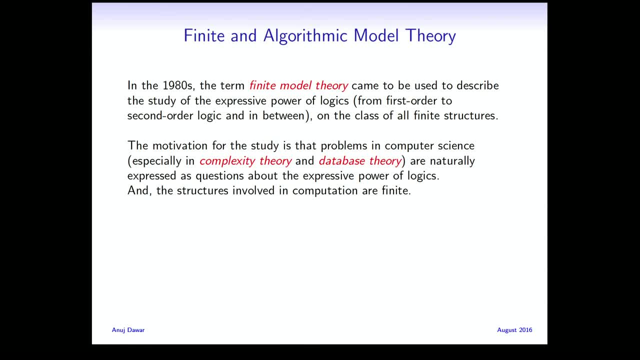 the structures involved in computation are finite and therefore we need to have specific tools for analyzing expressive power in the context of finite structures, And the tools from, say, classical model theory simply don't carry over. So there's a wide range of techniques, many of them algorithmic, and we'll look at this. 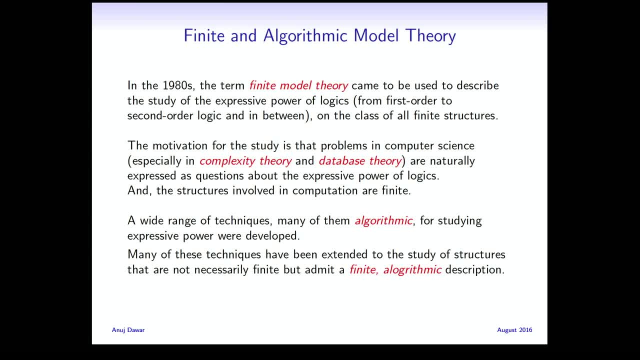 And many of these then extend beyond considering finite structures to structures which may be infinite, but typically which have finite or algorithmic description. They can be described By In some kind of formal way- Okay, Okay, Okay, Okay, Through finite descriptions and so on. 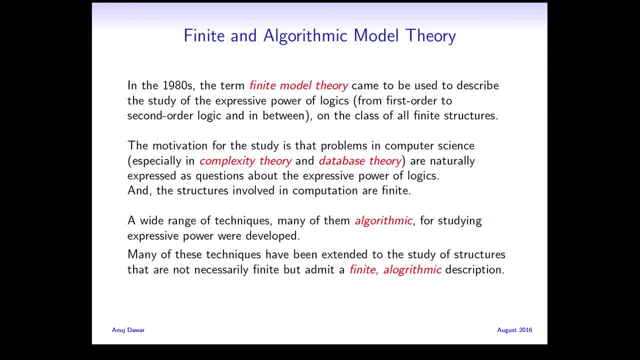 That's why we generally now talk of finite and algorithmic model theory. There's a lot to be said on this, but in this course of lectures I'll go I'll generally stick to finite structures and say very little about the extensions, as I said, because I'm 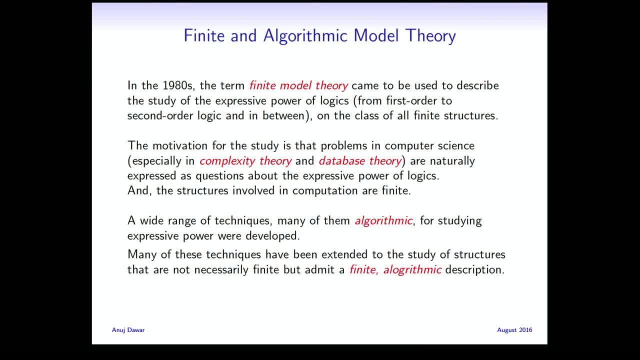 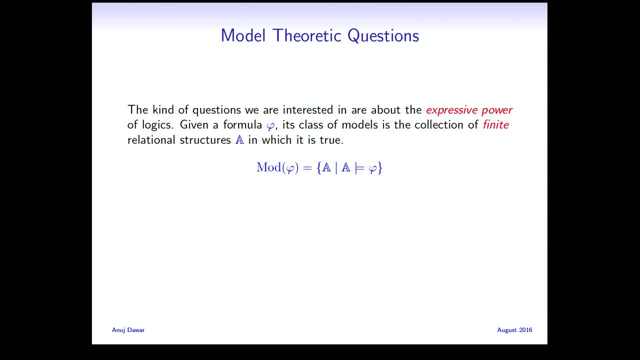 going to focus mainly on the, on techniques. Okay, So what do we mean? What do I mean by model theoretic theory? Okay, So we're going to talk about model theoretic questions, questions about the expressive power. So typically the kind of thing we're saying is: we have a formula and a logic. 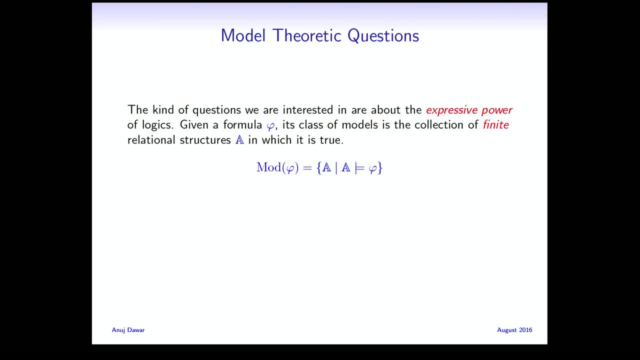 I'll make this all a little bit formal in just a little bit. And we ask about its class of models, say the class of finite relational structures. Now let's say this formula is in a relational vocabulary, has certain relations and constants, And so when I talk about the models of phi, I'll typically mean the collection of finite. 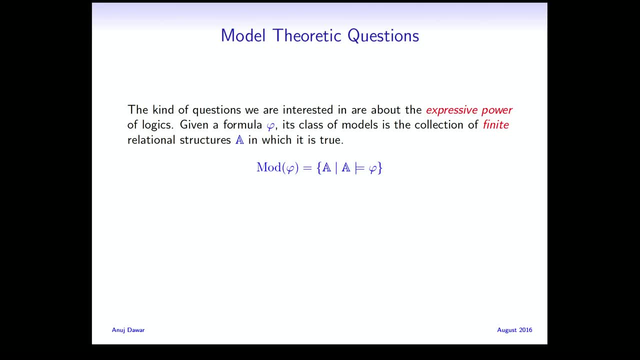 structures which satisfy it And we want to ask essentially what classes of structures are definable in this way. Okay, And I say in a given logic L, we will start with say first order logic, but then we'll consider variations of this. 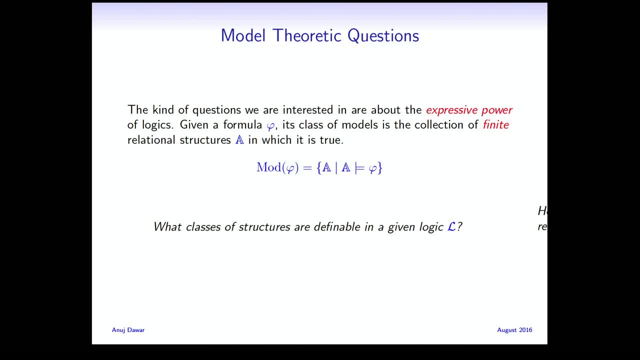 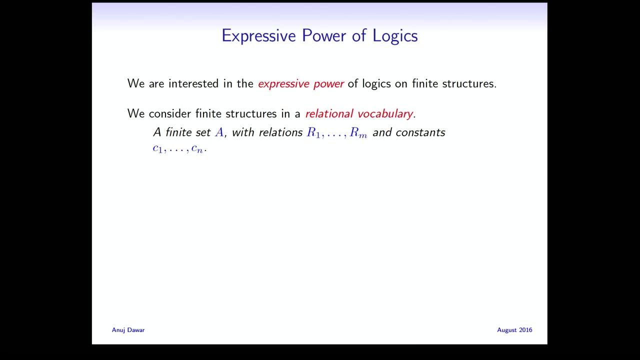 But this is the kind of definability question we're interested in. Something's gone wrong here. I'm not even sure what that says now, but I'm sure it was nothing important. Okay, Okay, Okay. So formally, a finite structure for us in a relational vocabulary is a finite set with 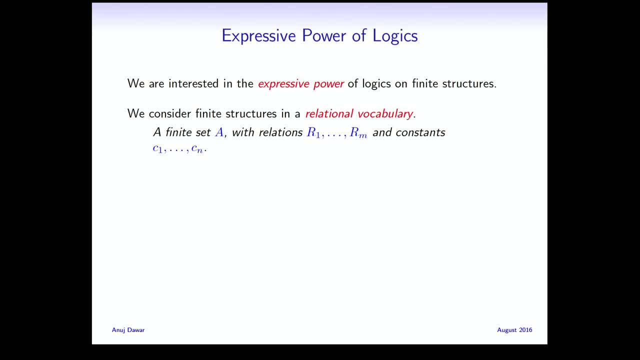 some collection of relations on it and some collection of constant symbols. So these constants are interpreted as elements of the structure. Each of the relation symbols comes with an associated arity as in it and is interpreted as a relational. So this is the relation of the suitability on this finite set. 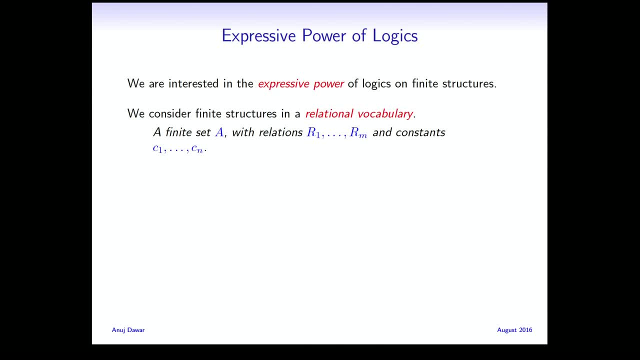 More generally, of course, you know you could consider function symbols. I'm not going to have function symbols around in my vocabulary in general simply because they make a lot of the statements that I'm going to make a lot more complicated to make. 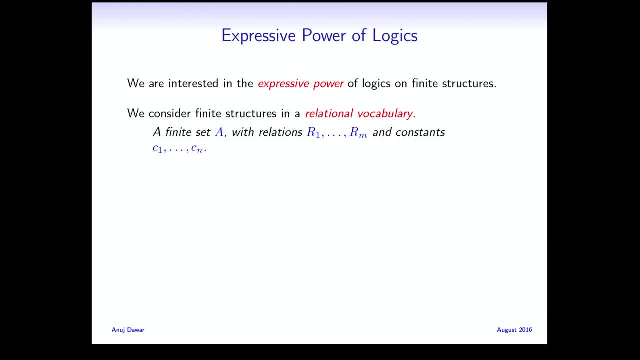 Okay, But without essentially changing them. I mean, they're all essentially true in the presence of function symbols, just a lot more complicated to say, So I'll just leave them out. You can ask me about that at the end if you'd like to know more. 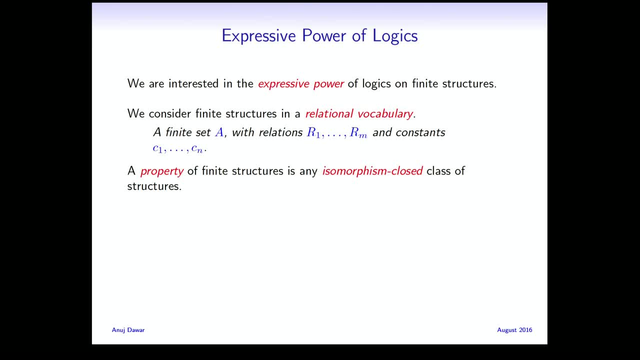 Okay. So when I say a property of finite structures or class of finite structure, I just mean any class of finite structures closed under isomorphism, right? So the We don't, Okay, We don't want to distinguish between structures which look the same. 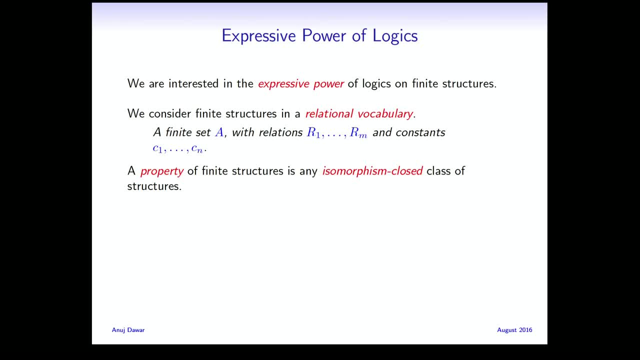 So isomorphic structures for our purposes are treated as the same And we're interested in certain properties of finite structures and we want to ask questions like: is a property definable or indefinable? So we ask for a given logic, L, for which properties P. 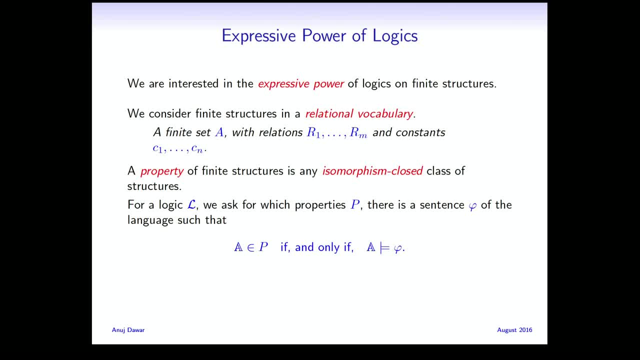 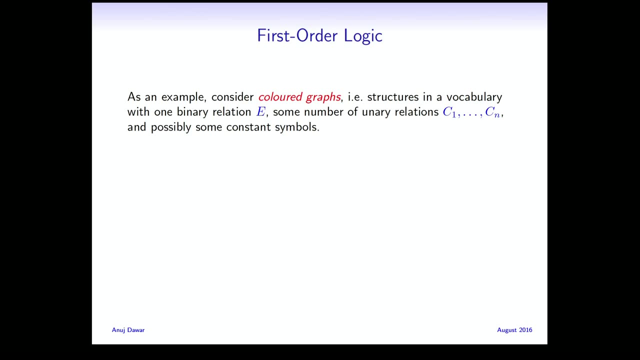 Is there a sentence in the logic which defines exactly this property? in other words, the structures that satisfy the sentence are exactly the ones that have the property P. Okay, That's our typical definability or undefinability question. So let's start with first order logic, simply because this is, I think, something which 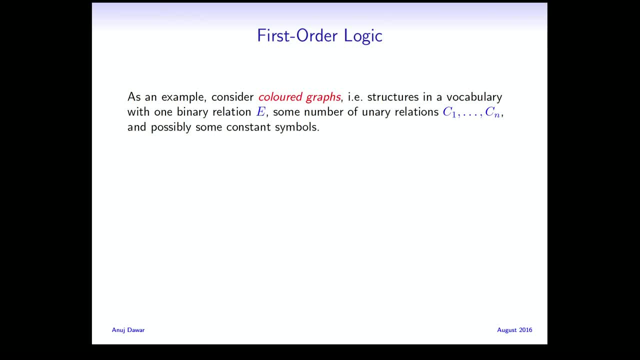 most people are familiar with. And as an example I mean we fix the vocabulary of certain relations and constants. So as an example, I'm going- And this will be a common One, running example I'll take through this course: Fix the vocabulary, let's say, with one binary relation and some number of unary relations. 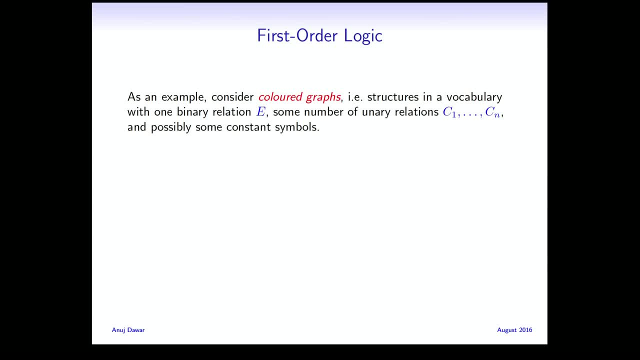 So this is R T 2. All of these are R T 1. And I call these things colored graphs. You can think of them as color directed graphs, right? So you have a set- We think of the set of vertices- a binary relation which we think of as the edge relation. 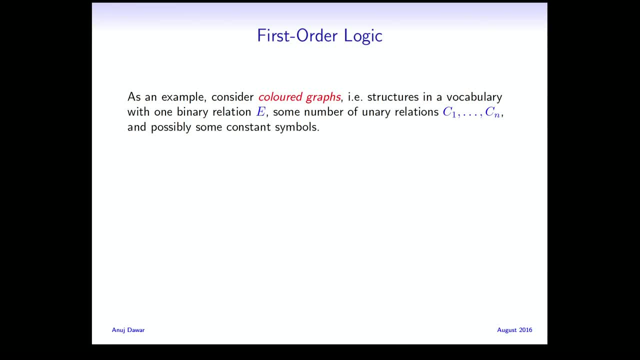 It's directed, because I haven't specified that it must be symmetric And we have some number of unary relations and I think of them as colors on the vertices of the Of the graph, Possibly some constant symbols. Occasionally I have constant symbols, So certain vertices may have distinguished names that I can use in my formulas. 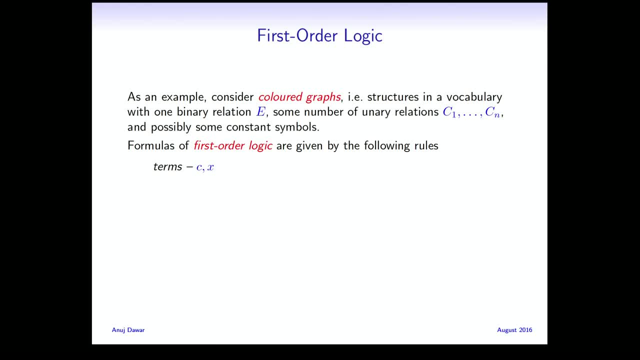 And now I formulate the first order logic through the following rules. We have terms. Any constant by itself is a term, Any variable by itself is a term, And these variables I think of as ranging over the vertices of the graph. We have a. 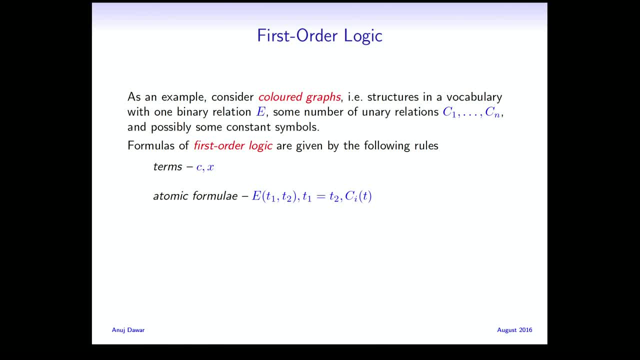 We form atomic formulas by saying that there's an edge between T 1 and T 2.. T 1 and T 2 are terms I'll always assume we have equality about. so we can say two things are equal And I can say that a certain 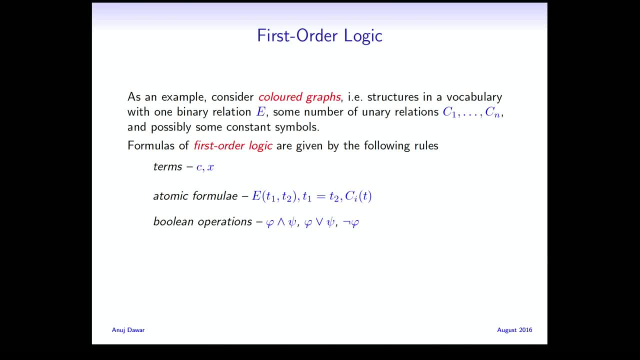 Some T has a particular color, Ci right. So those are our formulas. We close under the usual Boolean operations And under first order quantifiers. So these quantifiers, in our case, are ranging over the vertices of a graph. So I can say there exists an X such that phi. 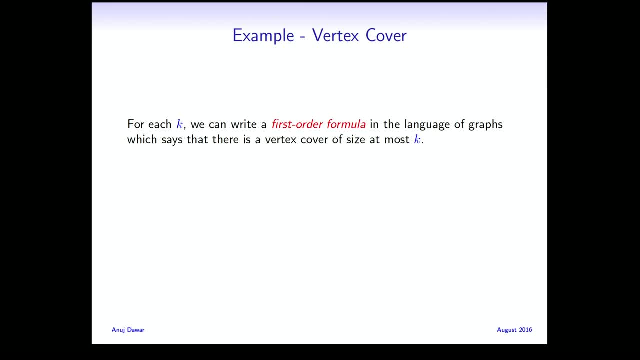 And for all X, such that phi. Okay, so here's a. I'll just write down an example formula of a kind of computational problem that we might want to express. Fix a positive integer K And I write a first order formula which defines those graphs which contain a vertex cover. 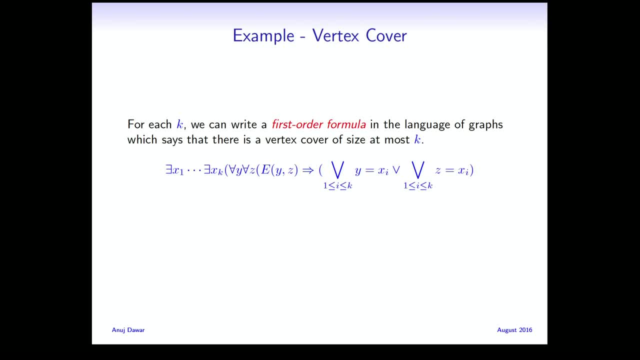 of size, at most K, right? So what is this? A vertex cover just says this. right, So there exists K elements. So is that For every Y and Z, if there's an edge between Y and Z, then either Y is one of the elements. 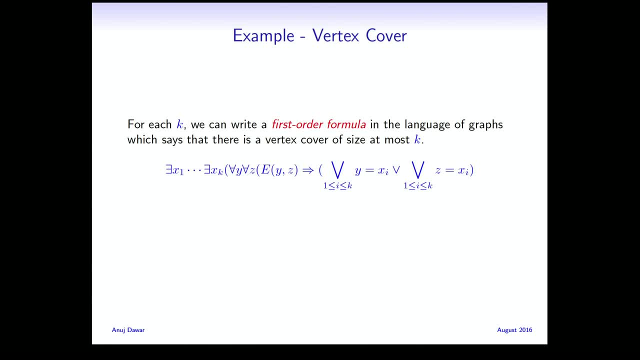 Xi, so that's a big disjunction over all values of I or Z is one of the elements Xi, So right for every edge. one of the endpoints is in the set X1 to XK. That's what it means for K elements to be a vertex cover. 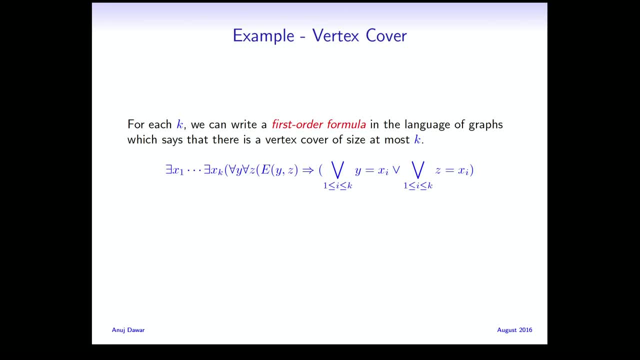 And so this formula is true when interpreted in a finite graph, if, and only if, the graph has a vertex cover of no more than K elements, No more than K elements, No more than K elements, No more than K, because you can interpret some of these variables by the same elements. 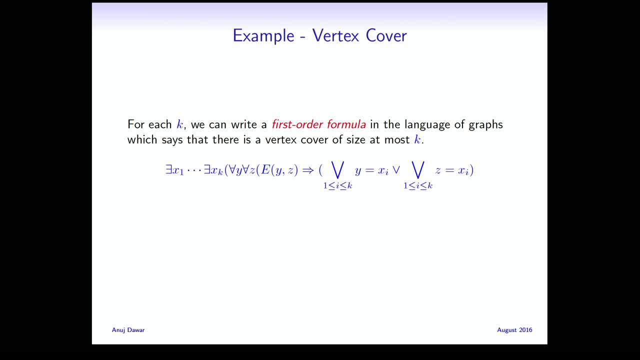 So this can be satisfied by a vertex cover smaller than K. OK, So quantifiers range over vertices of the graph. To pick another problem, say we want to say the graph is three-colorable Here. we can't do it, and we'll see why we can't do it as we go on. 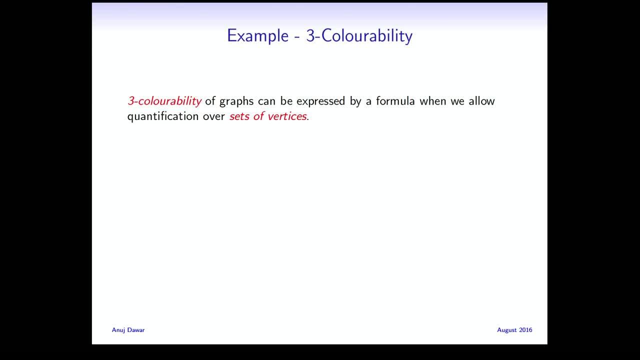 We can't do it with just A first-order formula, that is, formula in which the quantifiers range over the vertices of the graph, But we allow ourselves quantification over sets of vertices. then we can say that a graph is three-colorable. 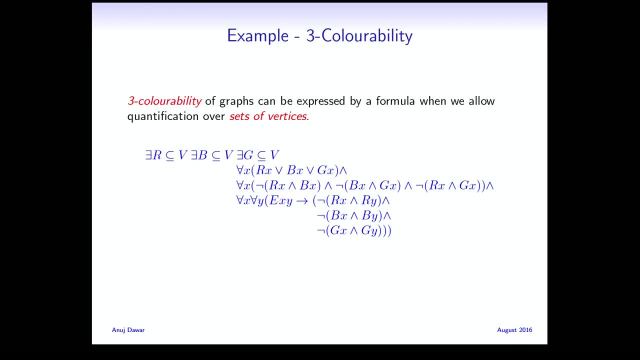 Right, So, as you can see. So this just- I mean it looks like a mess, but it says the obvious thing. There are three sets of vertices. I've written V here, but of course this is Well. I should have done that. 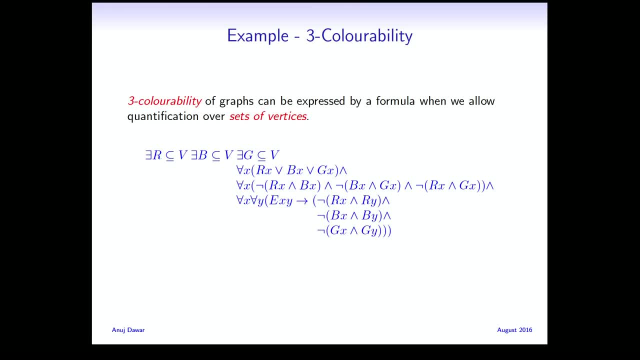 I should have done that. I should have done that, I should have stressed this out. There exist three sets: R, B and G. I just emphasized that. they're sets of vertices And every element is in one of those sets. 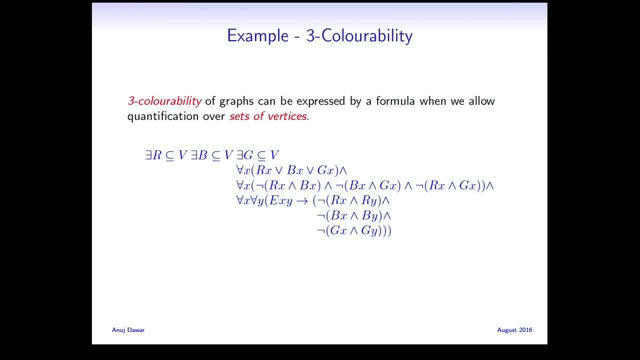 No element is in two of those sets And whenever you have an edge, the two endpoints are in different sets. OK, So that says there is a proper three-coloring of a graph Right Now. This is OK. So this slide is just a bit of a nod to classical model theory. 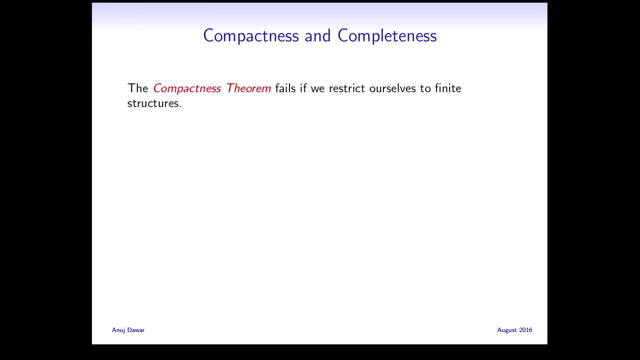 I said that. you know. finite model theory, at least, is named in reference to classical model theory, which studies the expressive power of logics in the context of infinite structures, And most of the methods available there are not very helpful when we talk of finite structures. 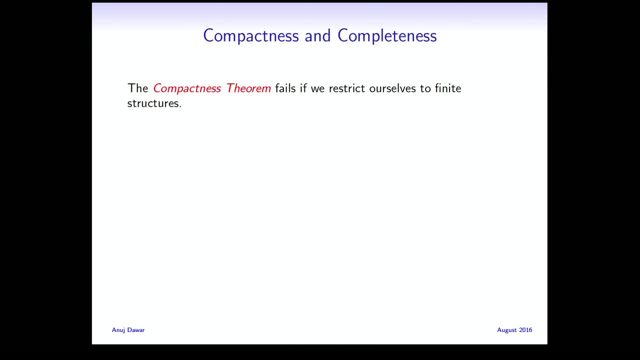 And I just wanted to mention this. The classical model theory rests on the foundations of two fundamental theories- The compactness theorem and the completeness theorem- And they simply don't tell us much when we restrict ourselves to finite structures. Compactness theorem fails in the obvious sense that you can come up with a set of sentences. 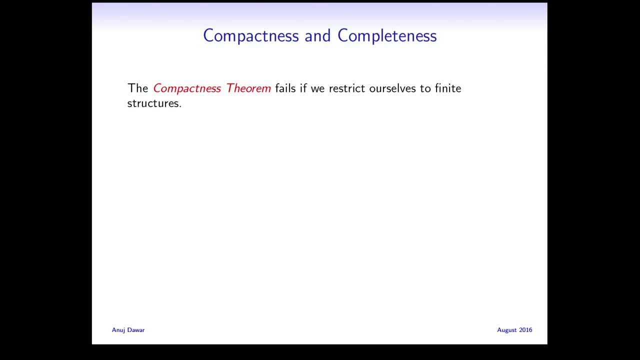 Every finite subset has a model in the sense of a finite model, But the whole collection is unsatisfiable because it has no finite model. That's kind of trivial to write And the completeness theorem fails in the strong sense that the set of sentences first. 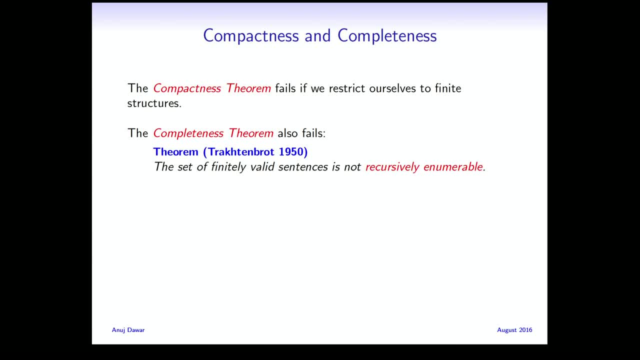 order sentences- the sentence of first order logic- which are finitely complex, Which are finitely valid- That is true in all finite structures- Don't form a recursively enumerable set. So there is no sense in which you can have a complete proof system for the finite validities. 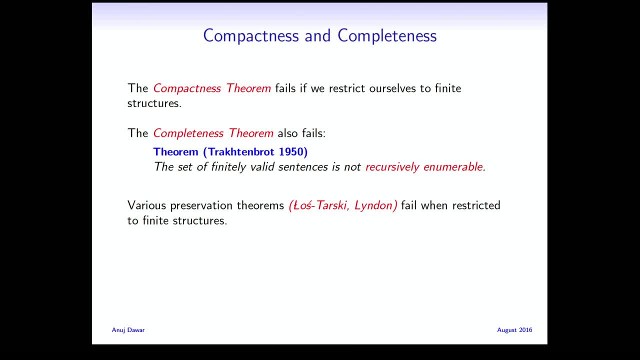 This goes back to Trachtenbrot. I said these are sort of the foundations of model theory in the classical sense. Various other things, for example preservation theorems of Wojtarski and Linden, fail when we restrict ourselves to finite structures. 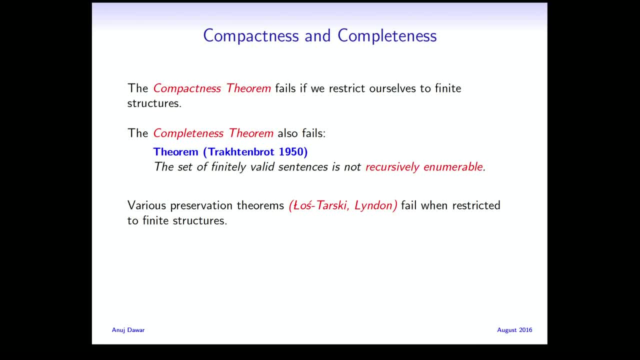 These are things which tell us that first order logics, syntactic properties of first order formulas are closely related to semantic closure properties of their models, And various finitary analogs of other foundational theorems also disappear. So the things on which classical model theory is built, the methods and the techniques- 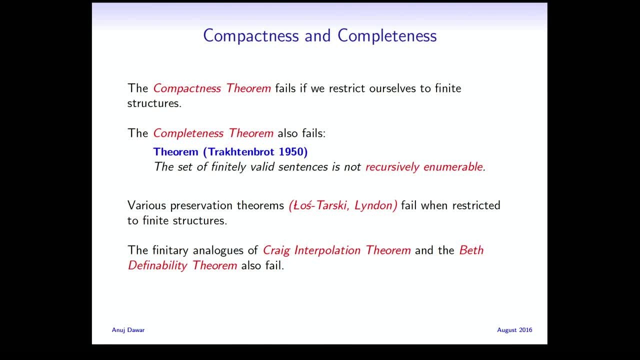 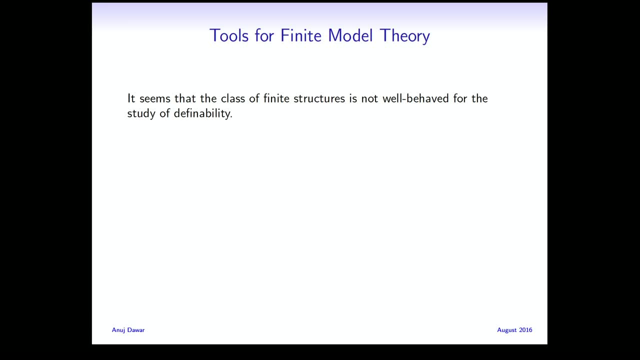 are simply not available for the sorts of things we want to study. OK, So what techniques do we have? So the class of finite structures in some sense is not well-behaved for the study of definability in the sense I mean. I remember back in the 90s having a conversation about this with John Barwise. 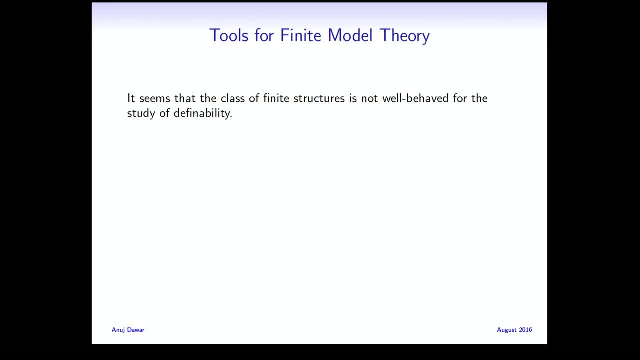 And he said: well, the class of finite structures is just not a natural class. Why would you want to consider it Right? But OK, What I want to now tell you is that there's now a slew of tools and methods to study expressive power of logic in the finite. 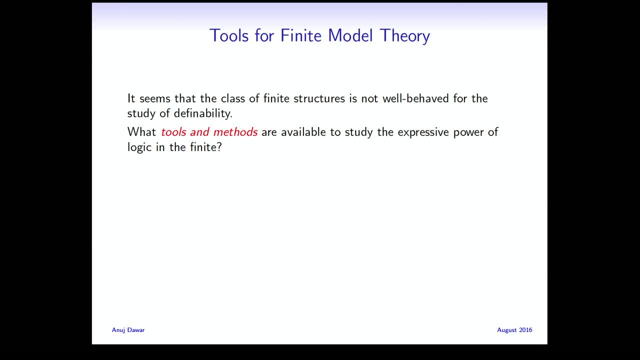 that I'm going to touch upon in this course, And a lot of these methods are essentially computational, algorithmic in nature. One which I'm going to start off with focusing on in this lecture is Aaron Foist-Ricey games, or model comparison games. 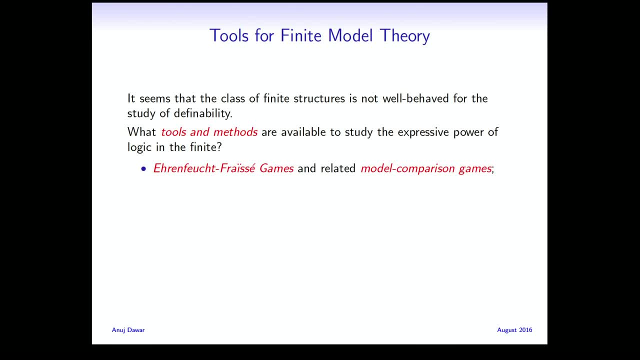 We'll see a few variations of these, And this is sort of a fundamental bedrock of analyzing expressive power of logic in the finite. It's just, in effect, just a different way of expressing when two things can't be distinguished in a certain logic. 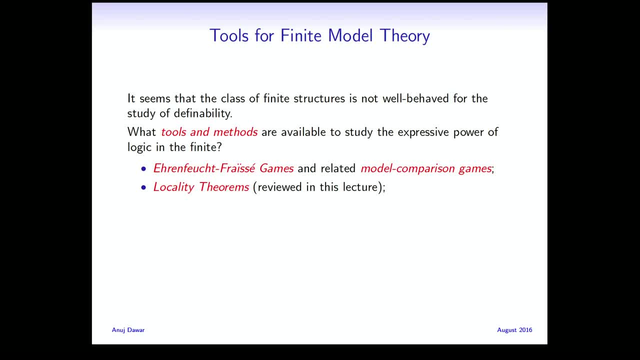 And then we build other tools on top of that. In particular, very useful are locality theorems, which I'll review by the end of this lecture and then pick up on in lecture three to see some maybe more sophisticated applications of these. There's automata-based methods for the analysis of logic. 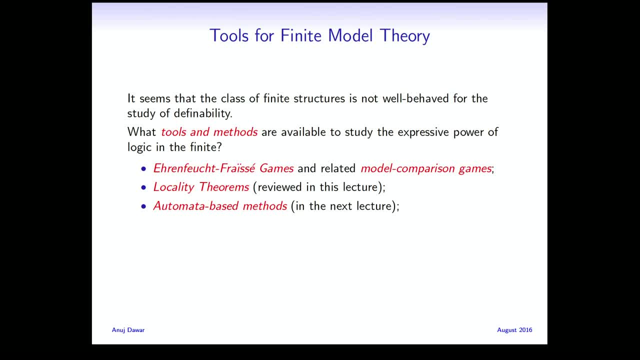 which will be the focus of the next lecture tomorrow. Complexity plays a big role. I mean you can Think of complexity. I mean a lot of. the motivation of finite model theory was to use model theoretic methods in the study of complexity. 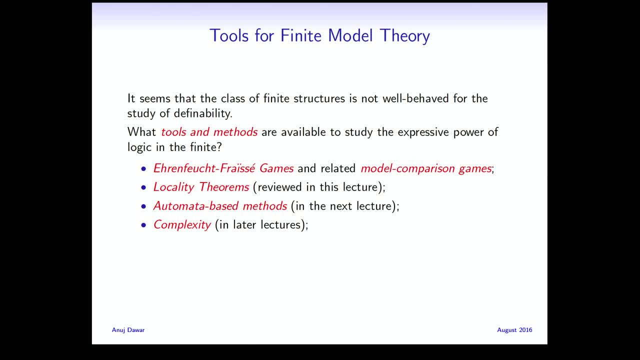 But of course the reverse is probably even more true. Using computational complexity as a way of analyzing the expressive power of logic has turned out to be very useful, And this will I say later lectures. It's a strand that will weave through a lot of what I have to say. 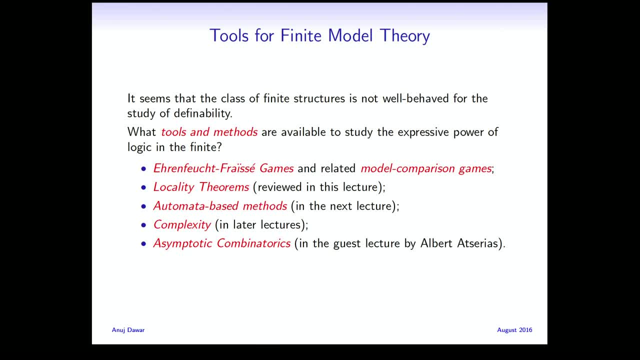 Asymptotic combinatorics. I should have mentioned Albert Atzerius will be giving a guest lecture on Thursday. He's part of this course and he'll focus on that. So these are. As I said, I've picked out five kind of thematic techniques. 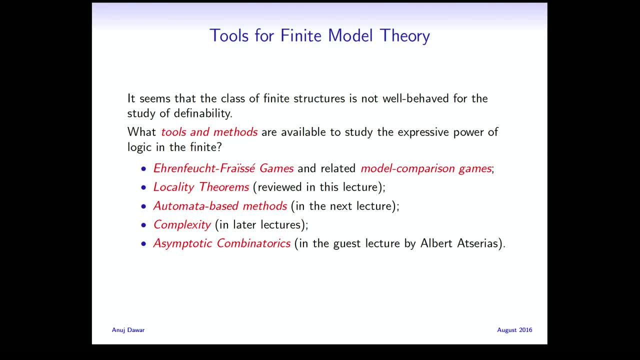 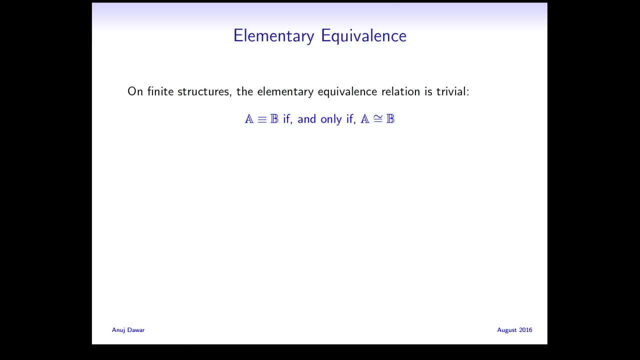 that are used for analyzing expressive power of logics, And this is how we sort of structure the course. Okay, So let's, I'm going to start and plunge in and talk about Aaron Fosch-Fresche games and related sorts of things. 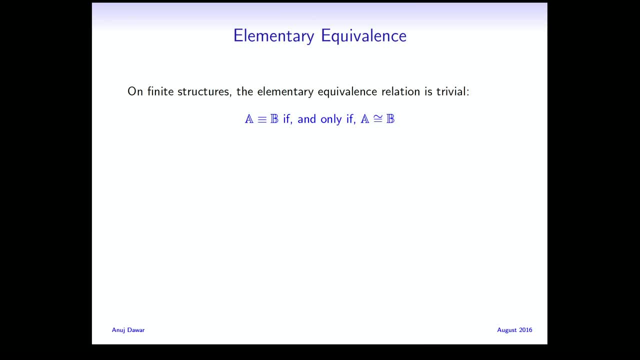 So the key idea is: The key idea is We have an equivalence relation on structures of elementary equivalence which says two structures are equivalent if they cannot be distinguished by any sentence of first-order logic. This is, again in classical model theory, the central. 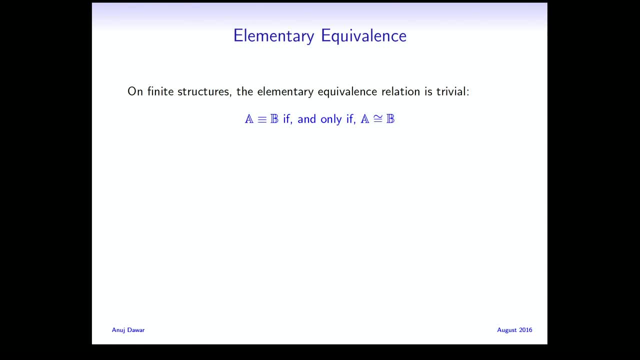 Well, in some sense the central object of study is this equivalence relation. You pick up a model theory book like the one by Chang and Kiesler, and I say: you pick a theorem at random from the book and it'll start with: let T be a complete theory. 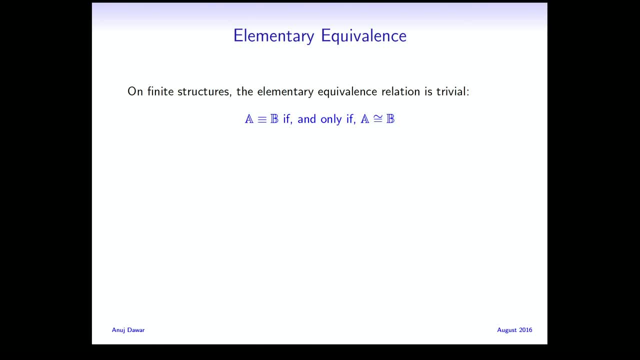 Which really means pick one equivalence class. in this equivalence relation You take the models of a complete theory. they form one equivalence class and then you go on to sort of say something about this On finite structures. this is an uninteresting equivalence relation. 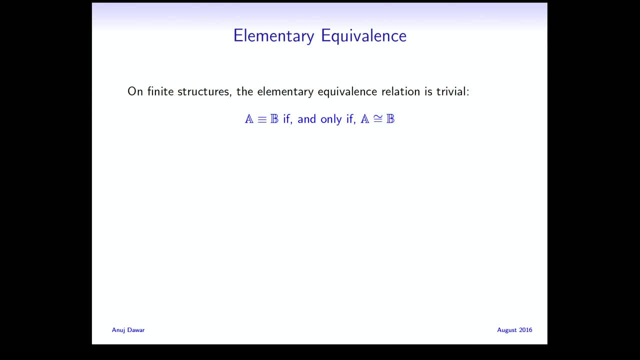 because it's the same as isomorphism. Two finite structures are elementarily equivalent if, and only if, they're isomorphic, and this is very easily seen. You start with a structure which has a fixed number n of elements and you write down a sentence. 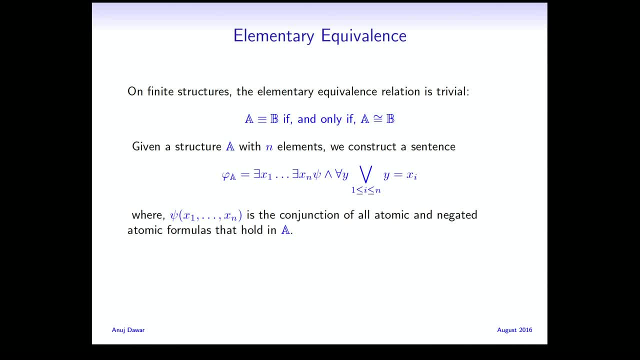 which describes it completely. You say there exists n elements and then you write a formula with the variables x1 to xn, which you know, having fixed a assignment x1 to xn to the elements of A, you just write down a formula. 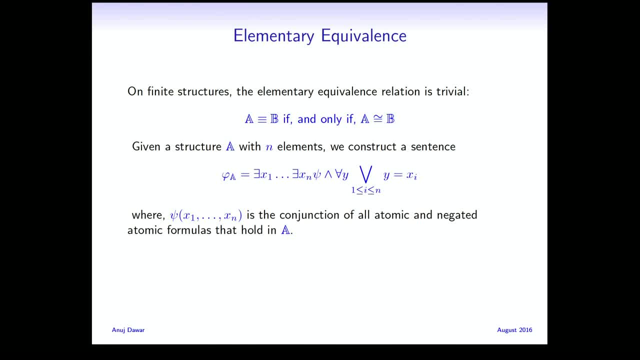 which says what things, what atomic formulas, are true and false, of those assuming a finite relational vocabulary here. So you just say everything there is to be said about the structure and you say that every element is one of them. Okay, and anything that satisfies this, of course. 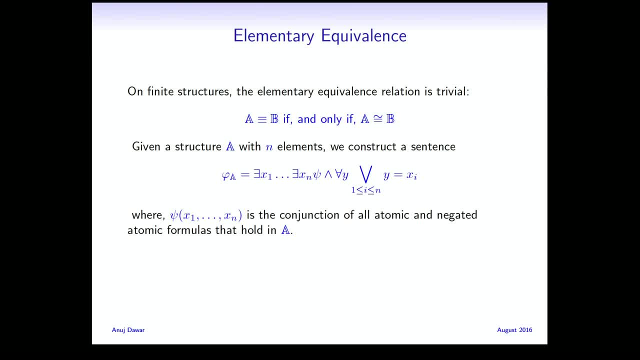 looks exactly like A. It's isomorphic to A, So anything that satisfies the same sentences as A is isomorphic to A Right. Anything that satisfies this sentence is isomorphic to A, So elementary equivalence is not very interesting in this sense. 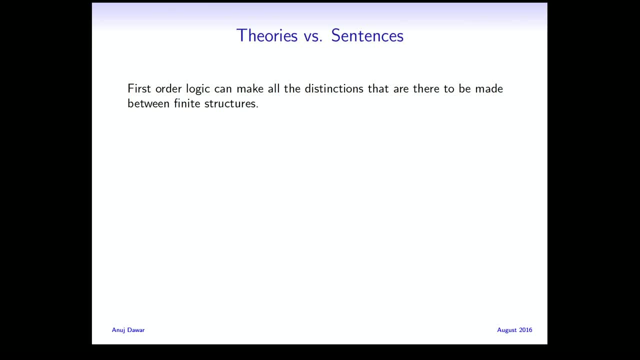 One way to understand what's going on here is, as I said, first-order logic can make all the distinctions that there are. It's not very hard to be made new in finite structures. That's what I just said on the previous slide. 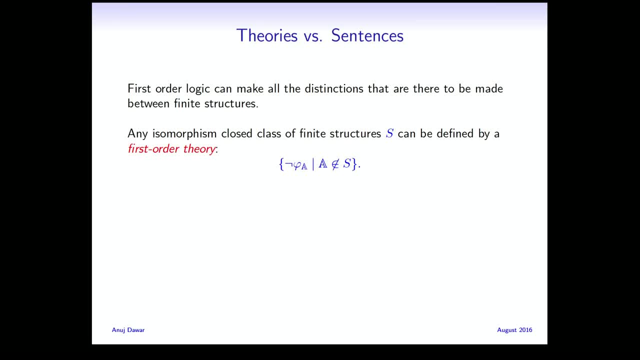 And so any property, what I call any property of finite structures, any isomorphism, close class, is defined by first-order theory. Okay, You take any property whatsoever, you take the sentences, take the structures which are not in S. 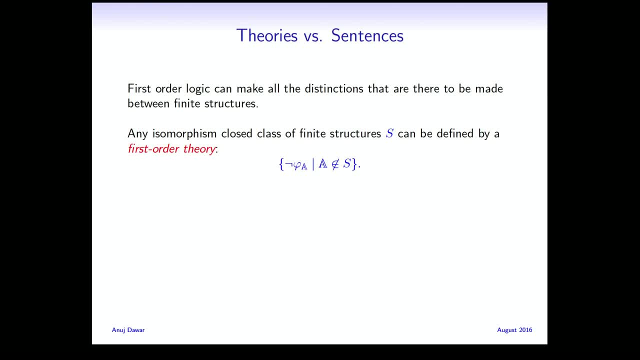 take the sentence which characterizes it, stick a negation in front and take the set of all of those. Anything that satisfies all these sentences is necessarily in S And so this theory, this set of sentences, sentences, defines us exactly. 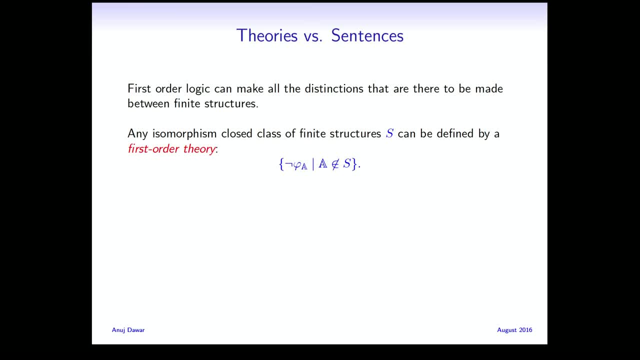 So classical model theory. being often interested in the expressive power of first order theories, that sort of aspect becomes uninteresting, And elementary equivalence is the right tool for analyzing the expressive power of theories If we want to understand the expressive power of first order sentences, in other words, 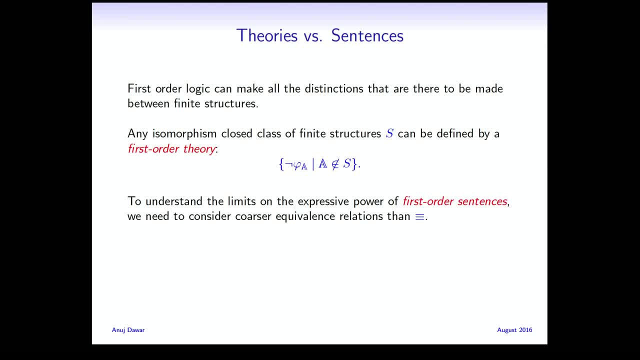 finite theories, finite collections of sentences. we need to consider equivalence relations that are coarser than this. Elementary equivalence just makes too many distinctions. We want to make fewer distinctions. I'm not just going to talk about the expressive power of first order sentences. 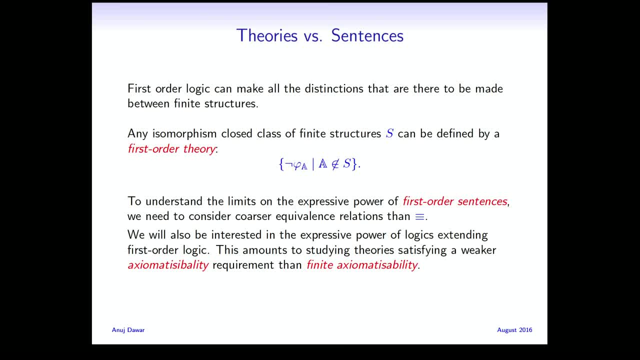 I'm going to also talk about logics which go beyond first order logic And one way of understanding. that is we're looking. we want to look at first order theories other than the finitely axiomatizable but limited in some other way. 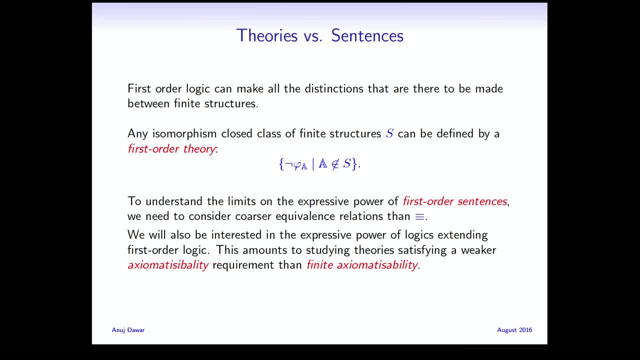 Right, And they we think of those as sentences in a logic more powerful than first order logic. You can unfold them into infinite first order theories, but they're sort of first order theories which are highly regular in some way or the other. okay, 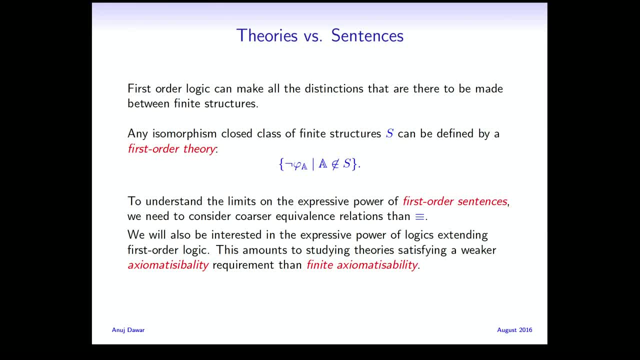 And that's what I say. it amounts to studying theory, satisfying a weaker axiomatizability requirement than finite axiomatizability. They're not necessarily finitely axiomatizable, but they'll be axiomatizable in some way, and we'll make that precise. 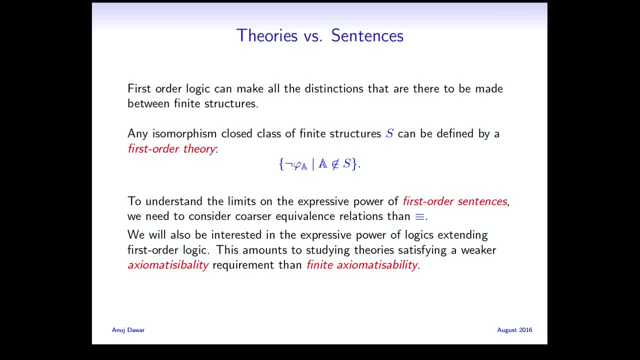 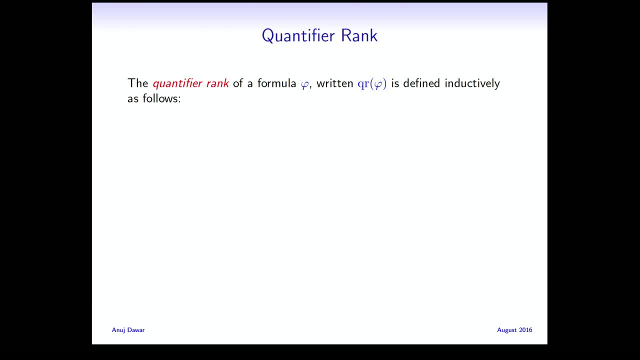 Okay, so now I'm going to talk about this: Understanding the limits of the expressive power of first order sentences by considering equivalence relations coarser than this one. So first focus will be on the quantifier rank of a formula. So we have a first order formula. 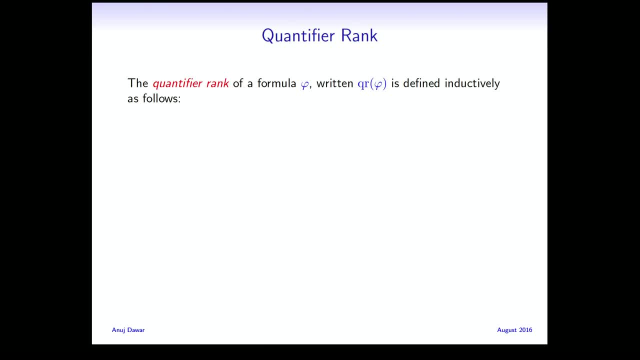 The quantifier rank is simply the. if you look at the formula, it's the maximum data. Okay, The quantifier rank is the depth of nesting of quantifiers inside the formula. I mean formally, I don't know that I need to go through this. I think what I've said. 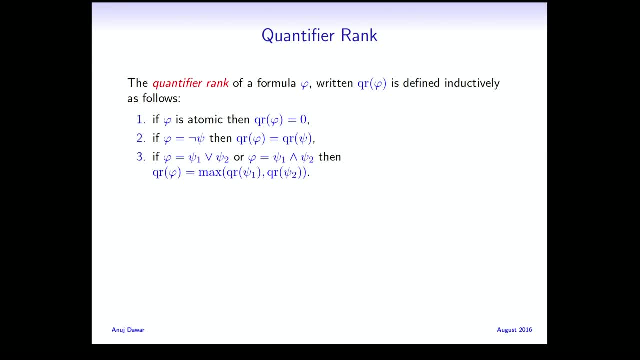 is enough for you to sit down and write down the formal definition right For atomic formulas: zero Boolean operations. you take the max and the quantifiers, increase the formula quantifier rank by one. Okay, I've already said this. 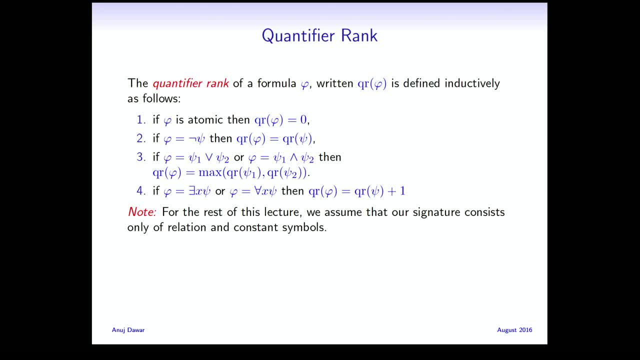 But maybe this is a good reminder. I said there are no function symbols, and this is really the crux of it. Okay, This is the reason why I said things would get complicated. We're going to use quantifier rank as a measure of the complexity of the formula. 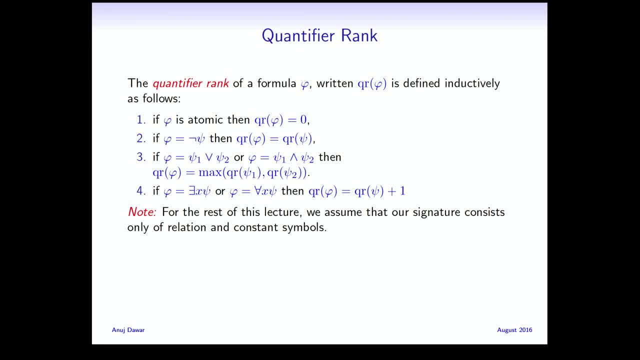 If we allow function symbols in our vocabulary, the nesting of function symbols inside each other introduces a complexity which isn't captured by this, and we would have to account for that separately. Effectively, functions and the nesting of functions are a hidden form of quantifier. 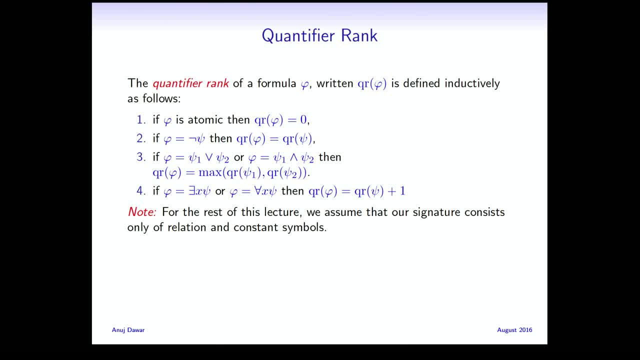 rank and by disallowing function symbols, it allows us to get a single measure, which is what we want. That's really the reason. Okay, With this proviso. okay, so now, if we have only relation and constant symbols, then in. 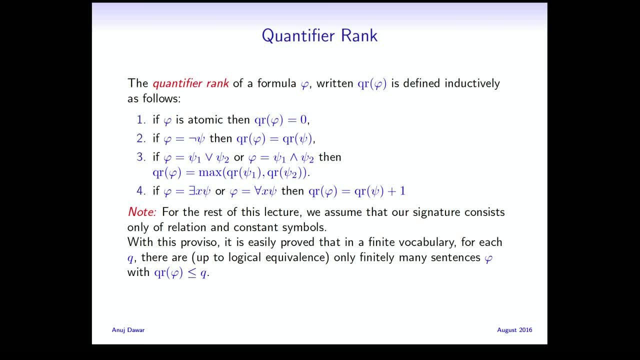 a finite vocabulary. once you fix the quantifier rank, there are only finitely many sentences you can write of that quantifier rank. Okay, This is a. So again, crucially Okay. This is false if you have function symbols, because you can nest the function symbols. 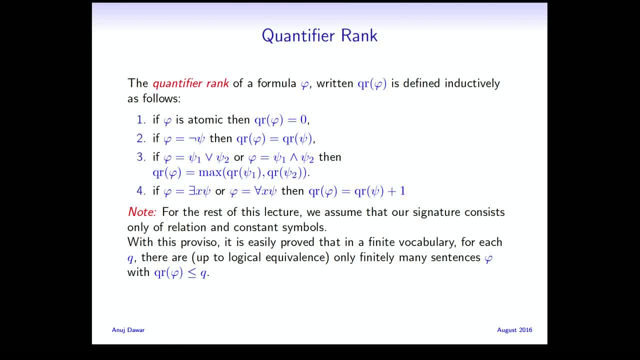 et cetera. Okay, There are only finitely many up to logical equivalence. This you can. I mean, I can, I think. leave it. it's an easy exercise to prove. Essentially, you prove by induction. you prove this by induction simultaneously for every. 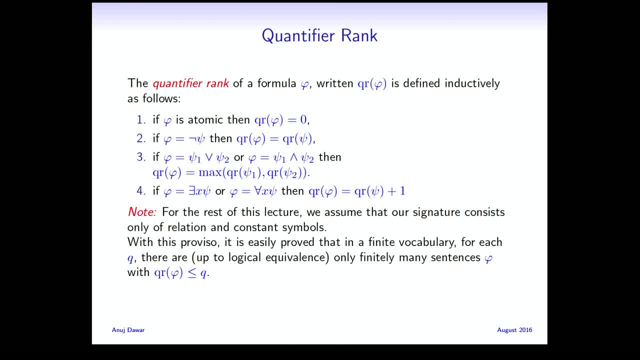 m, that the number of formulas with m free variables is finite. Okay, Right, Once you bound the quantifier rank, That's the. It's a kind of. You need to keep track of two things: the number of free variables and the quantifier. 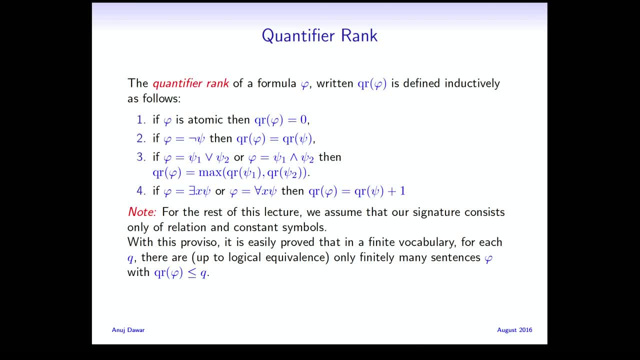 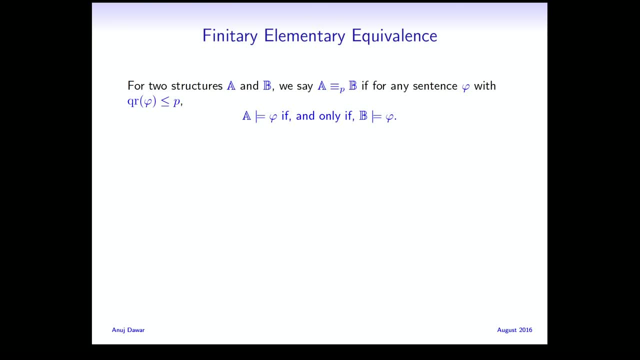 rank. Okay. So now we say two structures are equivalent up to p if they can't be distinguished by any sentence of quantifier rank at most p. Okay, I've gone to using from q to p. I thought I'd used p throughout, but 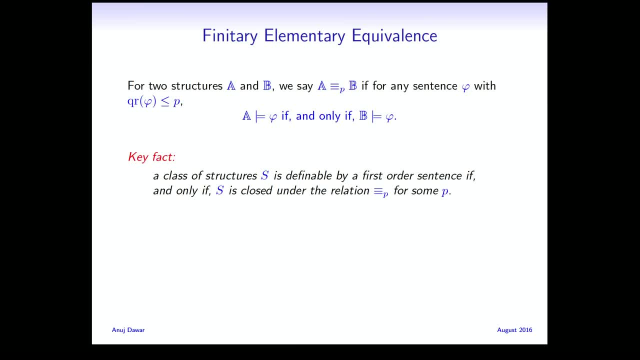 Okay, And now? this is in some sense the right notion for analyzing the expressive power of first order logic in the following sense: If a class of structures or some property is definable by first order sentence, it's closed under this equivalence relation for some p. 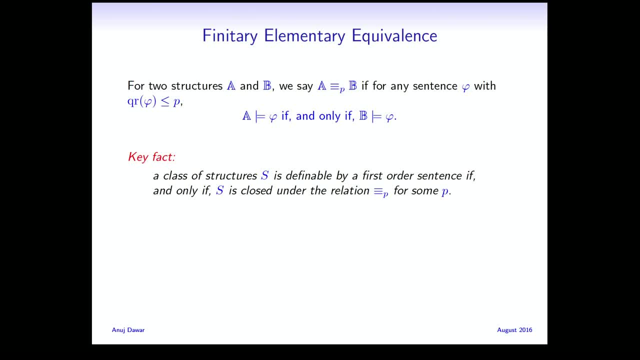 That's kind of obvious, because the first order sentence has some quantifier rank, p, and so s must be invariant under that p. But the converse is true. But the converse is true as well. Any property closed under this equivalence relation for some p is definable by first. 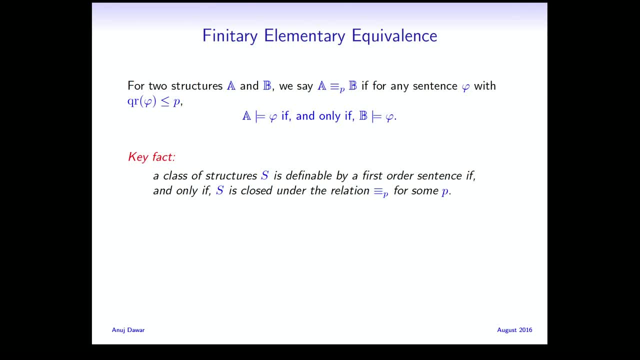 order sentence. And this follows from what I had on the previous slide, namely there are only finitely many sentences of quantifier rank p up to equivalence. So this thing actually has finitely many equivalence classes. For every pair of them you can find a sentence that distinguishes them. 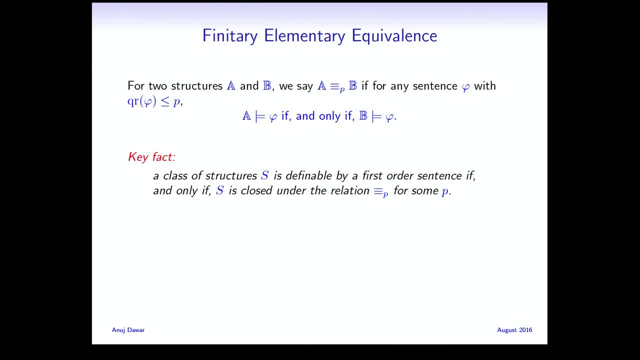 Boolean combinations of those will define every collection of equivalence classes. And that's all there is to it. But we can say a bit more. Just like we constructed for a structure, a single sentence which describes it up to isomorphism, you can also construct a single sentence which describes it up to p equivalence. 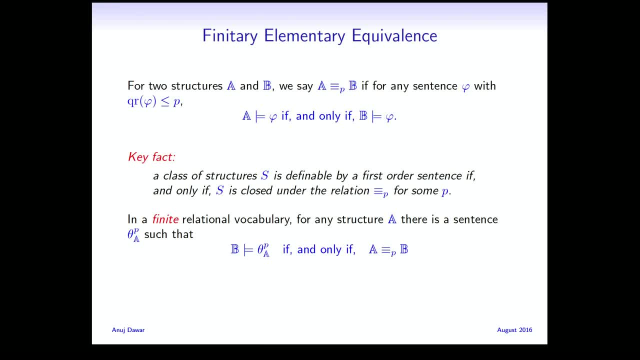 That again pretty much follows from the fact that each equivalence class is defined by a sentence, which is what I just said, And that's this: This is the sentence which describes the equivalence class of A. I mean, you can give an explicit construction, but this is enough for our purposes. 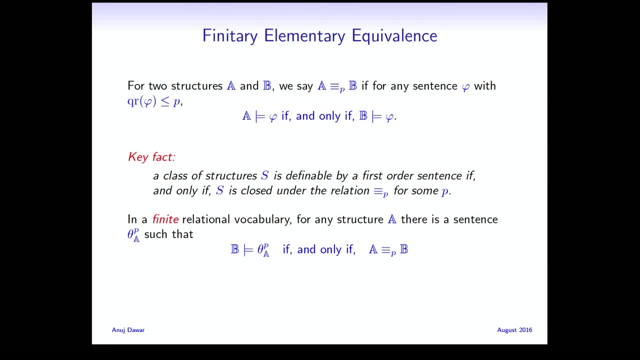 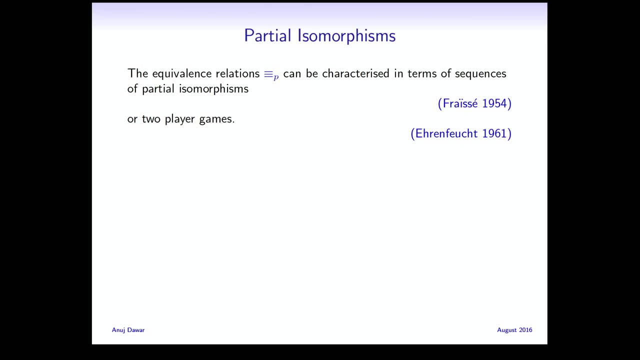 OK, So now I'm going to focus on this a little bit and see how we can say something meaningful about this equivalence relation and deduce that certain things are not definable in first order logic. Right, That's the aim. now, The essential thing is, these equivalence relations have a nice characteristic. 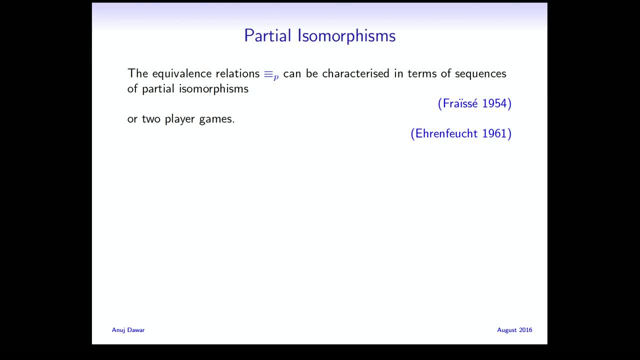 They're not defined in the first order logic Right, That's the aim. now, These equivalence relations have a nice characterization, which was first given by Freise back in 1954, in terms of sequences of partial isomorphisms. Aaron Feucht gave a description of this in terms of two-player games, which is nice, and 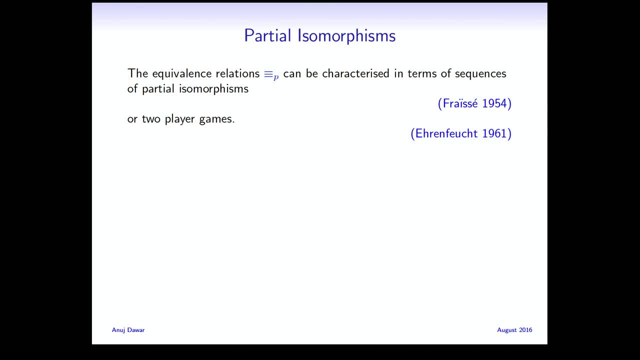 perspicuous and makes it a very useful tool. So let me just explain what it is. A partial isomorphism from A to B is simply an injective partial function Which takes the interpretation of any constant to the same constant in the other structure. 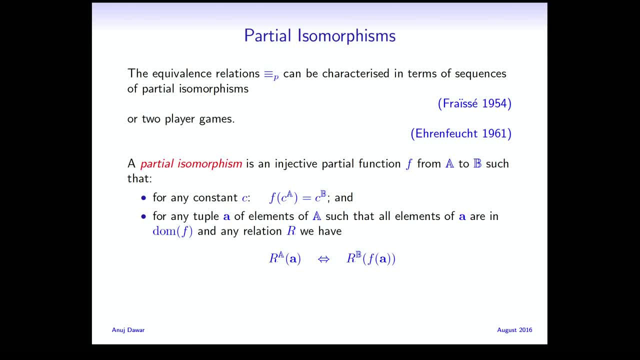 and preserves all the relations. So whenever we have a couple of elements of A, all of which are in the domain of this function, then that A is that couple is in a relation on the left. if, and only if, its image is in the relation on the right. 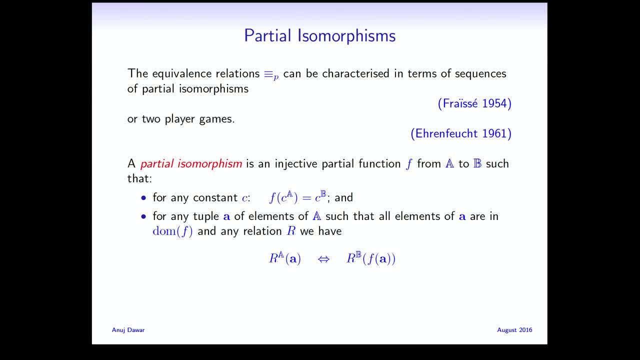 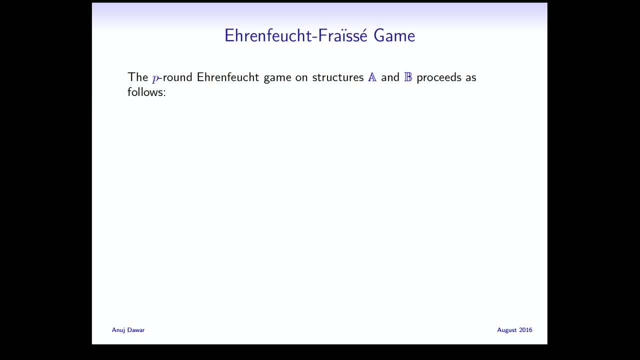 OK, So it's just what you'd expect. It's an isomorphism on the domain of F, Right? OK, So this is the requirement that F is defined for all the constants. let's say So what do we have? 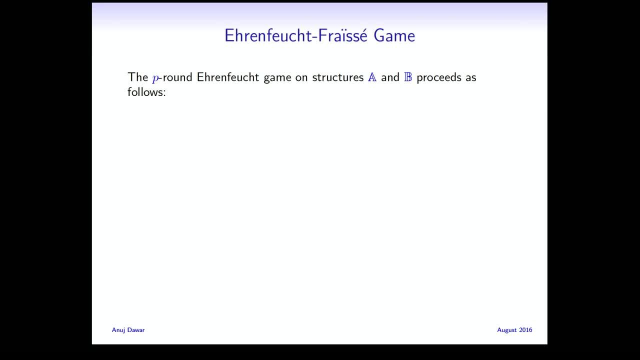 So I'll give you the game characterization of Aaron Feucht. The P round Aaron Feucht game on structures A and B is as follows: We have two players- We now call them spoiler and duplicator- And the idea is we have a pair of structures, A and B. 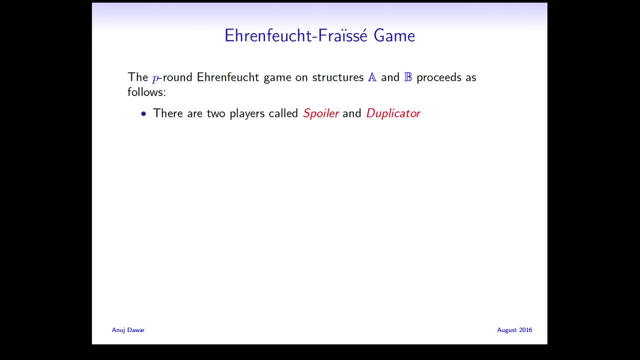 Spoiler claims that these structures are A and B. These structures are different. Duplicator claims that they are the same And they play a game to see which one of them can establish their claim. At each round of the game, spoiler chooses one of the structures, for example B. 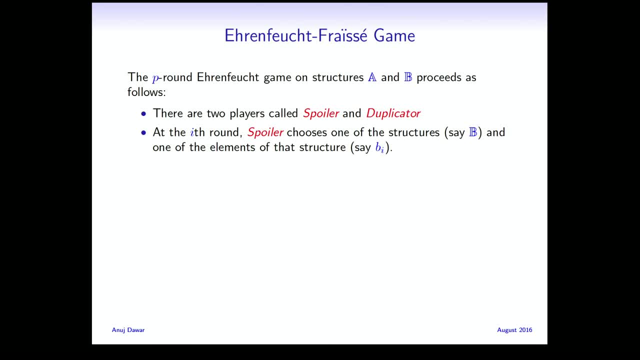 Right, And the choice is made at each round. So in different rounds you could choose a different one And an element of that structure. call it B sub i, the i subscript- i referring to the round- And duplicator has to respond with an element of the other structure. 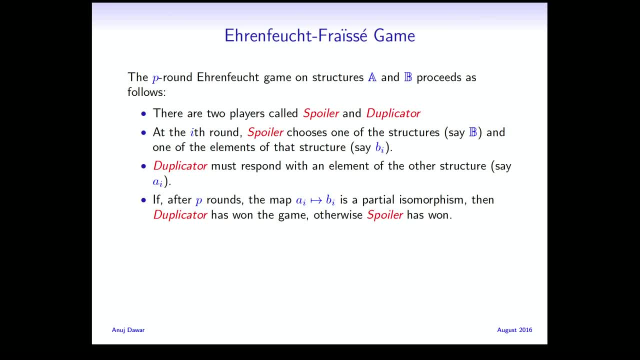 And you look at after P rounds. you look at the map which takes the element chosen at the i-th round in A to the element chosen in the i-th round in B, along with the map on the constants, which is fixed anyway. 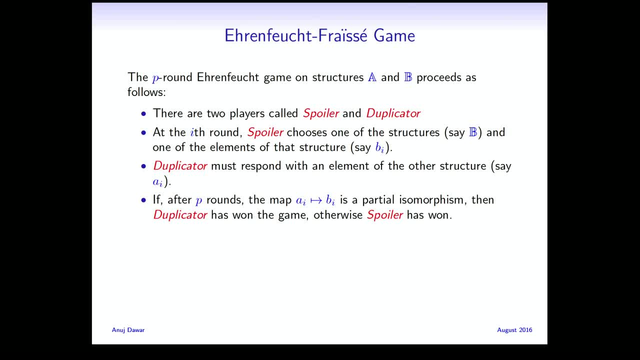 If this is a partial isomorphism after P rounds, then duplicator has won. Spoiler has failed to demonstrate a difference between them. But it's not a partial isomorphism. Spoiler has won. Spoiler has demonstrated that the two structures are different. 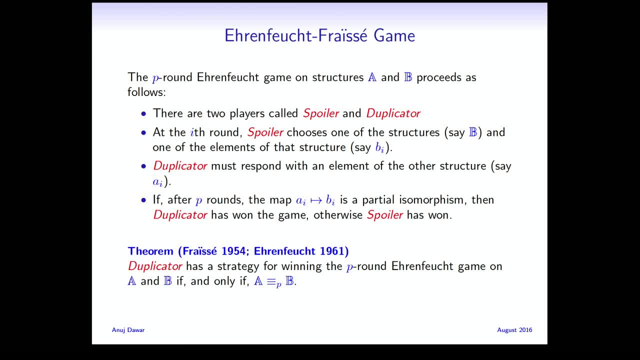 So that's the idea, And the key thing that connects this with what we had before is that duplicator has a winning strategy if, and only if, the two structures are equivalent. So this is not very difficult to prove, given what we have already. 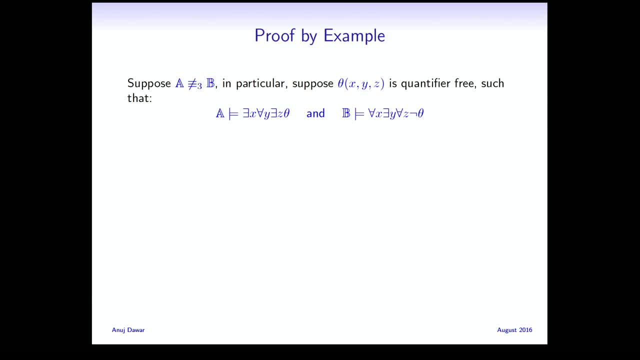 I have on the next slide what I call proof by example. just to give you the connection, Suppose- and this is only doing one direction of it- Suppose A and B are not three equivalent means. they're distinguished by some sense of quantifier rank three right. 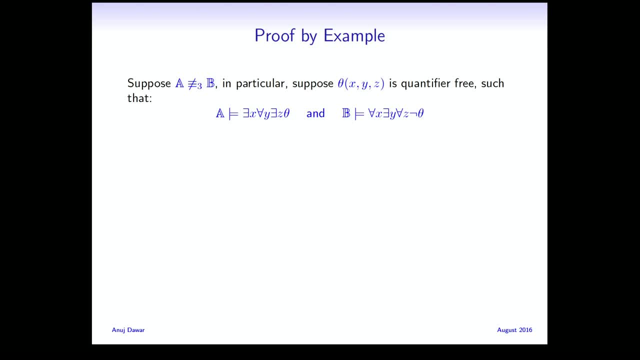 And let's say that sentence is of the form: there exists x for all y, there is a, z, theta, where theta is some formula involving those three variables, then it's true in A and false in B. So I want to say that this sentence essentially describes a strategy for spoiler. 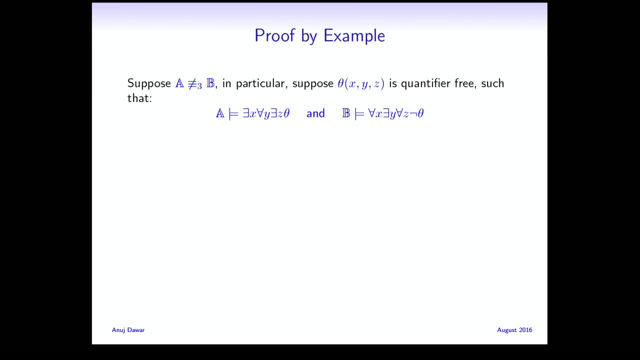 to win the three round game. What's the strategy? Well, round one. this existential is satisfied in A and not in B. Therefore, spoiler chooses an element of A which satisfies it. Duplicator has to respond with some element of B. Necessarily, this element will not satisfy. 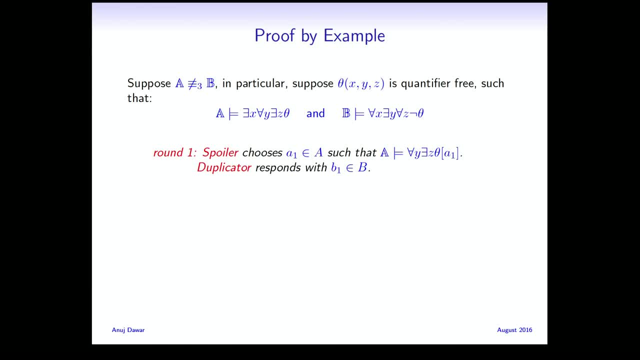 this existential because B satisfies the negation of that. Now, whatever B1 chose, Because of this universal this, there exists x for all, z not theta, is true of B1.. And so spoiler, in the second round, chooses a witness for that existential right. 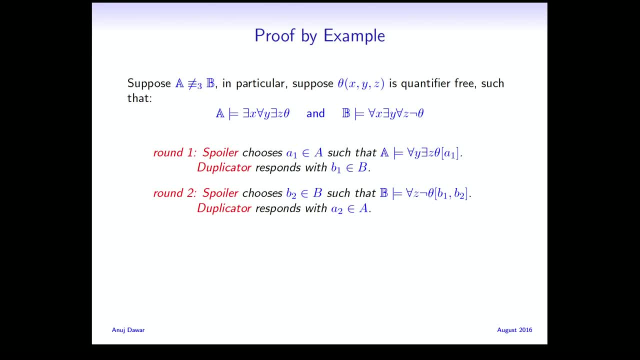 So chooses a B2, which satisfies for all z, not theta, B1,, B2.. Duplicator has to respond with an element of A, Necessarily because of this universal. there exists z, theta is true, And so spoiler chooses a witness for that z in A which satisfies this and clearly. 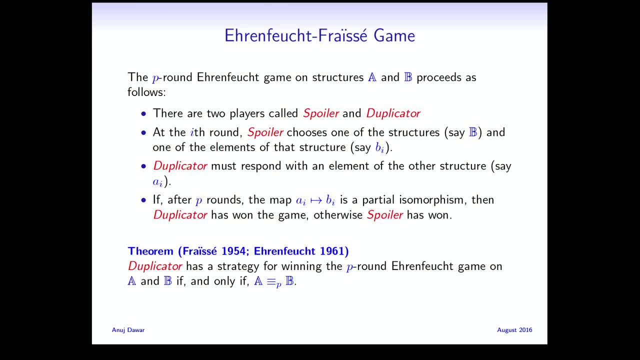 spoiler has lost. You generalize this to arbitrary first order formulas and that gives you one direction of this. if and only if The other direction crucially uses again the fact that we are in relational vocabularies and we have finitely many sentences. 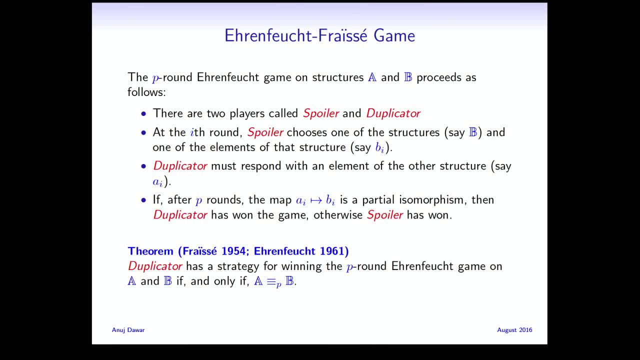 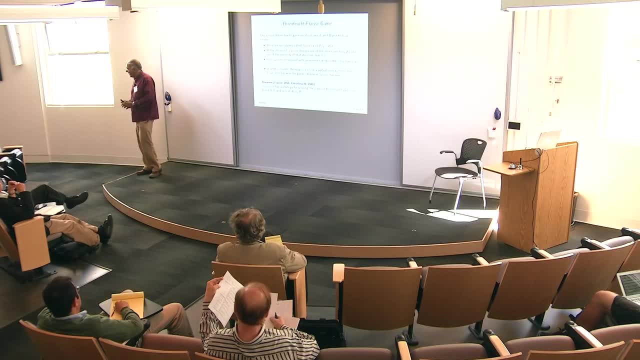 Peter, Is it obvious that it's still true when the formula is not in pre-next form? Well, is it obvious? It is true, Yeah, obvious. How big is the strategy you just described? Well, it's not that big. 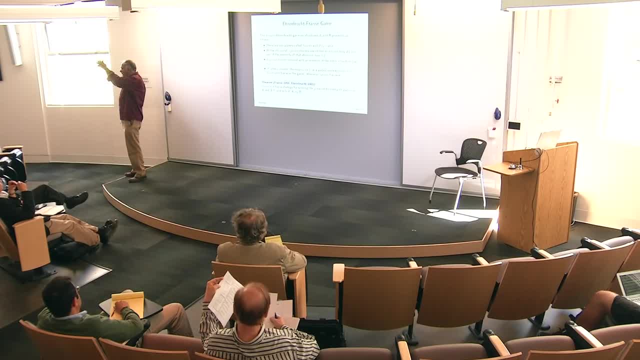 It's not that big. It's not that big. So the strategy essentially, exactly. The point is so: what happens when you have a conjunction or boolean combination of formulas? If you have a conjunction that's true in one and false in the other, you just pick the. 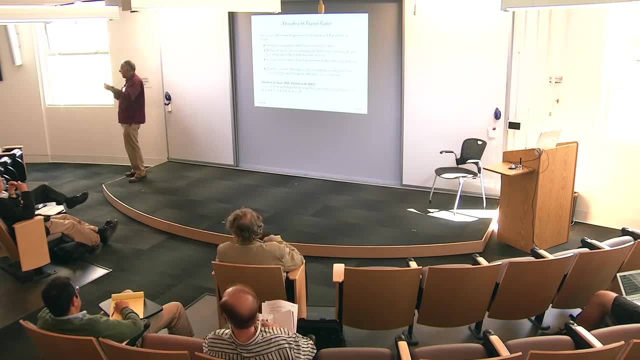 conjunct that is true in one and false in the other. Same thing with disjunctions And with negation. you sort of flip the roles of the two. But you're absolutely right, because putting it in pre-next normal form changes the quantifier. 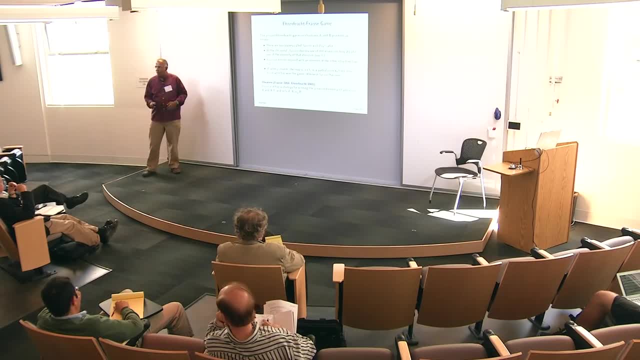 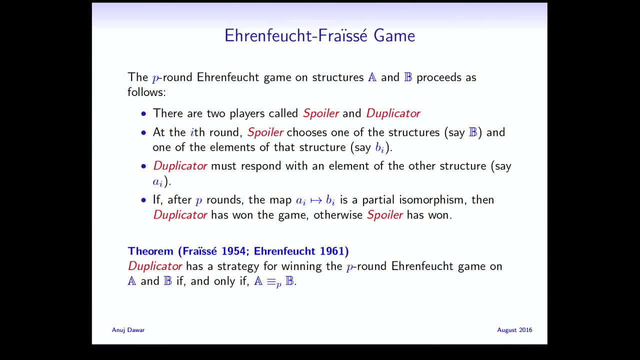 rank. So it is important that we consider, in general, formulas that are not in pre-next normal form. So, as I said, my example shows one direction. In fact, that's the direction of this that we will be using, the direction that says: 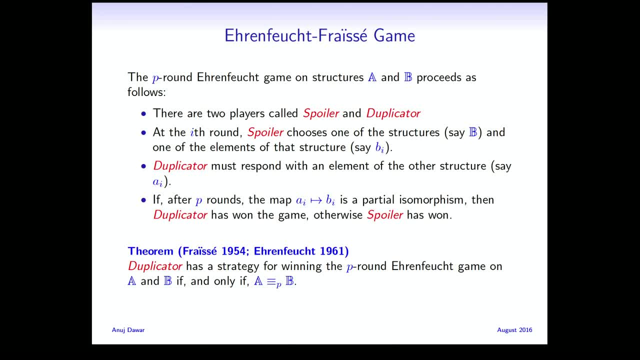 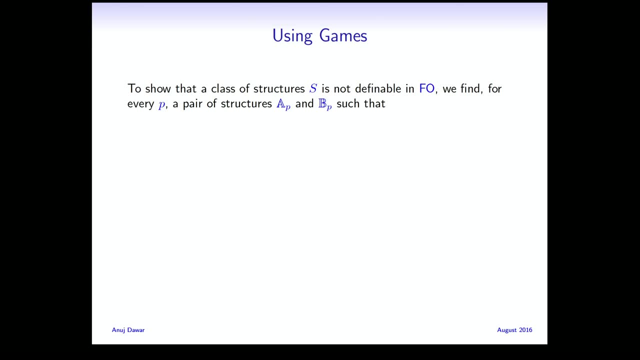 if the two things are distinguished, then spoiler has a winning strategy. So in other words, if duplicator does have a winning strategy, then they are indistinguishable. OK So, OK, So how do we use this? So we want to show that a class of structures is not definable. 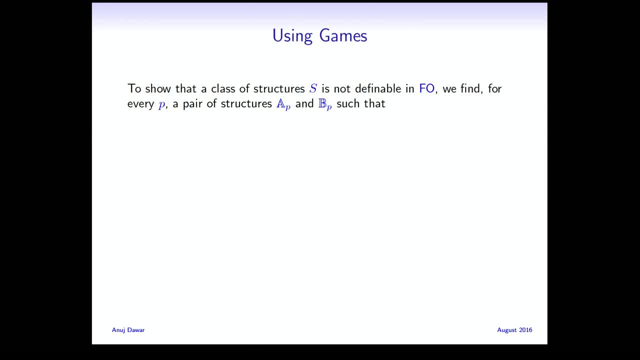 We have to find for every p, every positive integer p, a pair of structures which are distinguished by this property s but not distinguished by p equivalents. In other words, we demonstrate that duplicator has a winning strategy in the game, in the 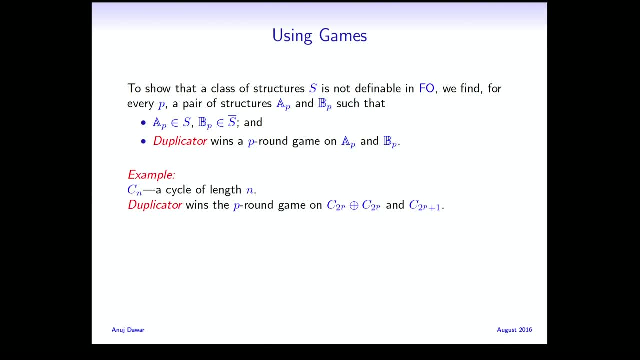 p-round game played between these structures. OK, So I'll give you an example. now Let cn be a cycle of length n. This is a graph. OK, So cn just denotes a cycle of length n. And now I consider two structures. I'll call it ap and bp. right? 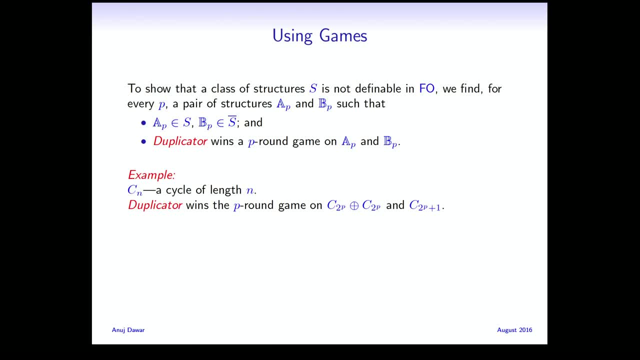 And ap is two cycles, disjoint union of two cycles, each of size 2, raised to the power p Right. So dp is a single cycle of size 2 raised to the power p plus 1.. OK, OK, So I claim, and I'll give you the argument on the next slide, that these two are p equivalent. 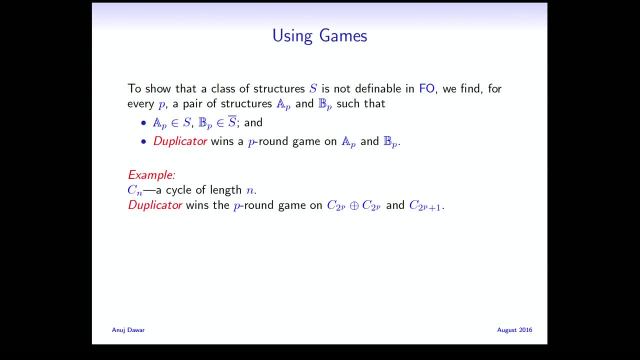 OK, So duplicator has a winning strategy for p rounds of the game. I'll give you the same reason, So I'll give you the answer. So it's less than 0.. So duplicator has a winning strategy for p rounds of the game. 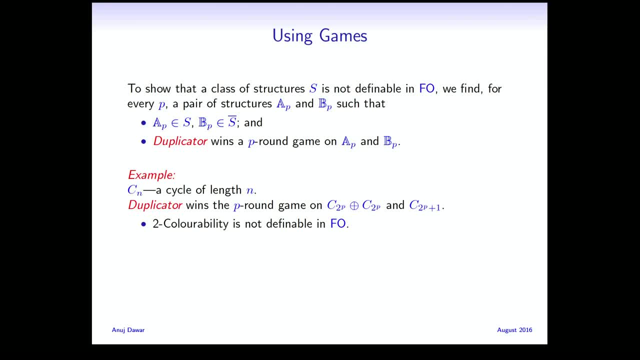 And this is a two color ability. For example, we get two color abilities. two color abilities are not definable in first order logic Graph. two color ability because two color ability is the same as the existence of a cycle of odd length. 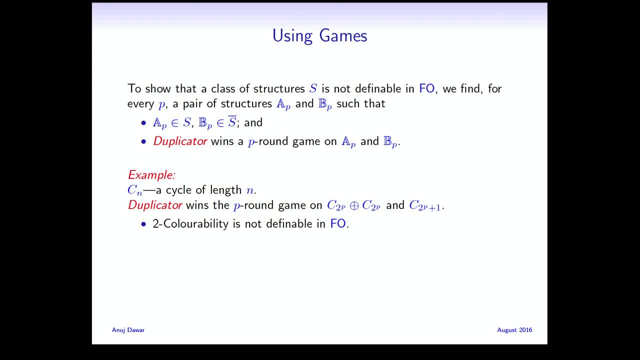 This graph has no cycles of odd length, but this one does Right. So this is two colorable, this is not So. two color ability is not definable in first order logic. Having an even number of elements is not definable in first order logic, simply because this graph 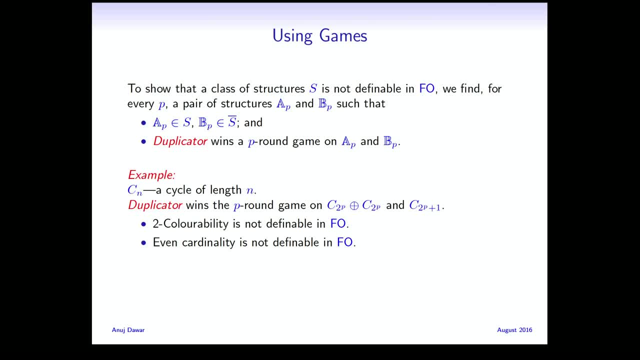 has an even number of elements and this one doesn't elements and this one doesn't right Connectivity property of a graph being connected is not definable in first-order logic because this graph is connected and this one isn't okay. So all of these follow from this one example. So, as I said, they're distinguished by these. 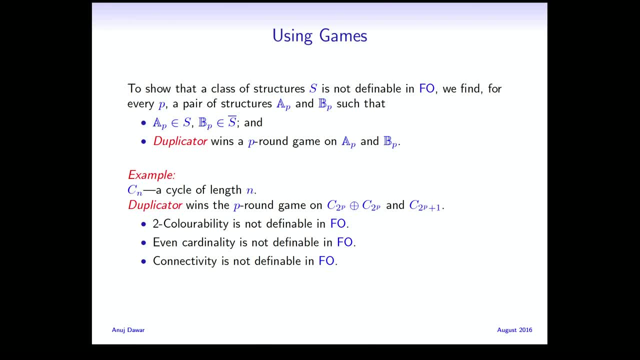 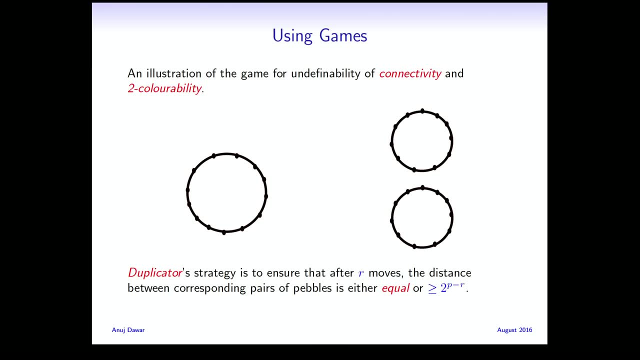 properties, but not distinguished. For any fixed P, we can find a pair of structures which are not distinguished. okay, So why is it that these two are P equivalent? We have to describe a strategy by duplicator and I've summed up the strategy in these two. 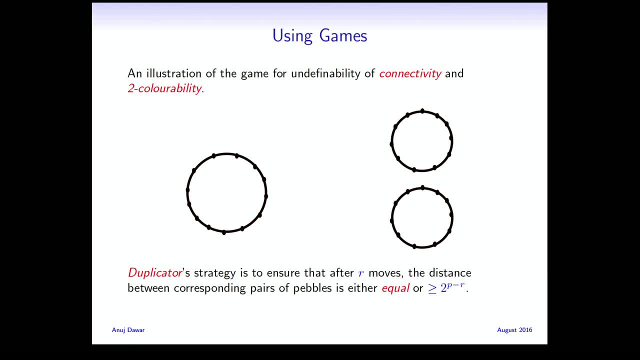 lines at the bottom. Duplicator strategy is to ensure that after R moves of the game have been played, we have to maintain a partial isomorphism for P moves, remember. So duplicator strategy is that after R moves have been played, the elements that have been picked in the 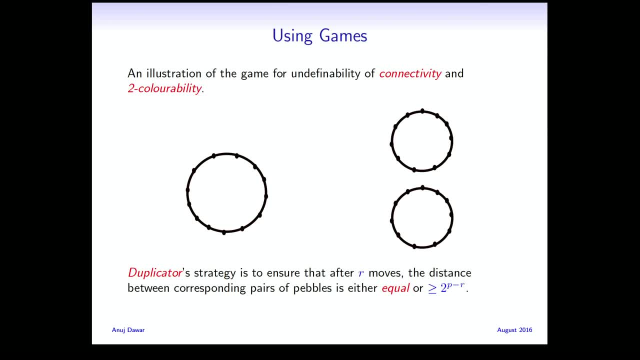 two structures, their distance, The distance between them. the graph, theoretic distance is either equal or bigger than 2 raised to the power of P minus R. okay, So the idea is: spoiler picks an element, duplicator responds with an element. For the first one, it really doesn't make any difference, They're. 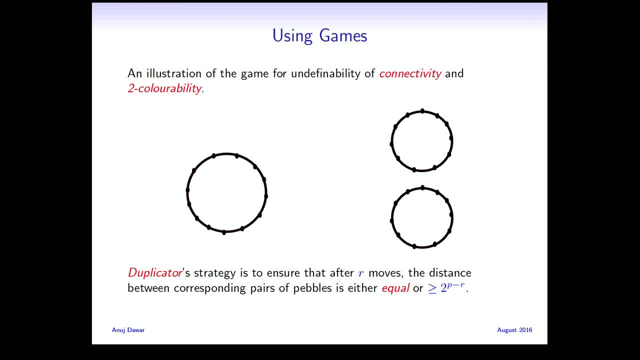 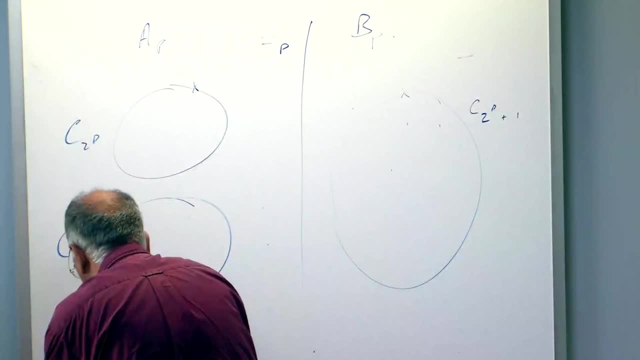 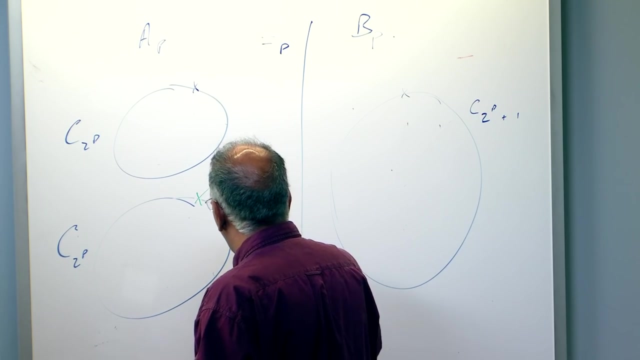 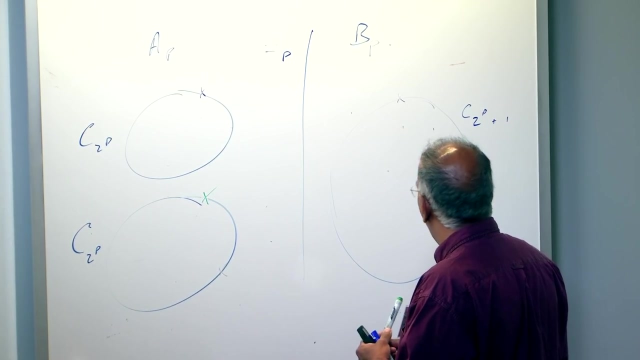 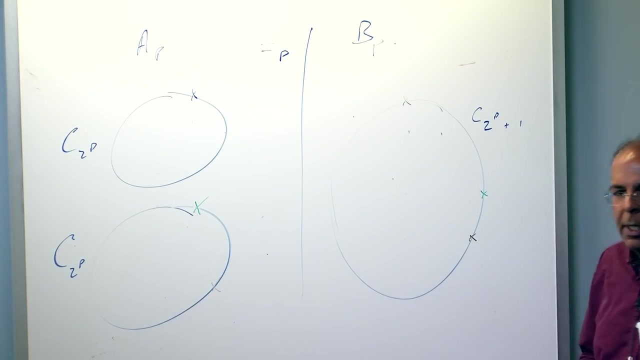 all interchangeable. Now, after some number of moves, you have, Let's say, these were three elements picked in three different rounds. So, And these are the ones chosen by duplicator in, or these are the ones chosen in B in response Duplicator. 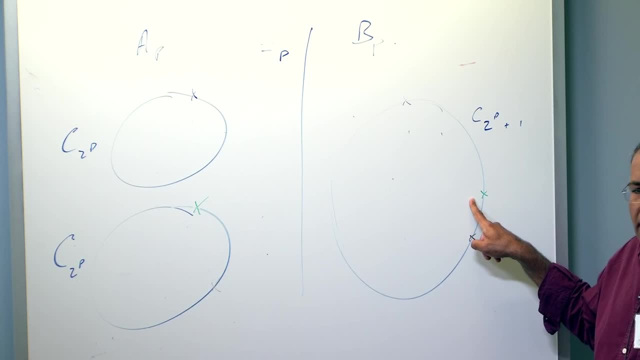 strategy is if the distance between two elements- And we can also repeat that by duplicating the distance between the two elements, by duplicating the distance between the two elements, by duplicating elements- is bigger, sorry, is smaller than what's happened here. oh, is smaller than. 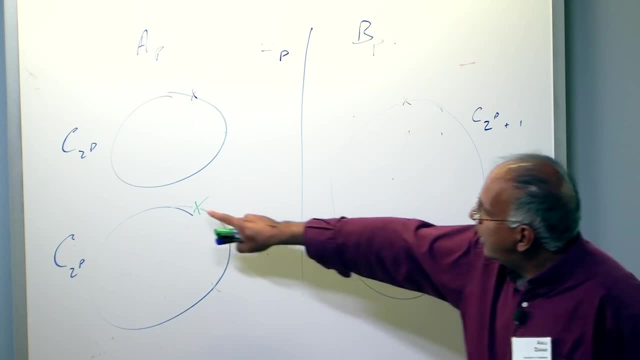 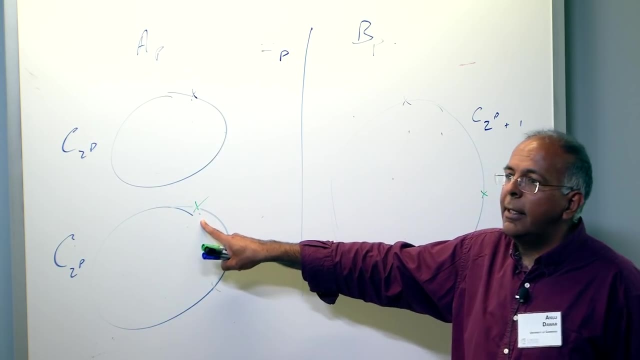 2 to the p minus r, then the distance over here is the same. So if this distance is small, then this distance is exactly the same as that. But if the distance is big, like here, it's infinite- then this distance is also big, bigger than 2 raised to the power of. 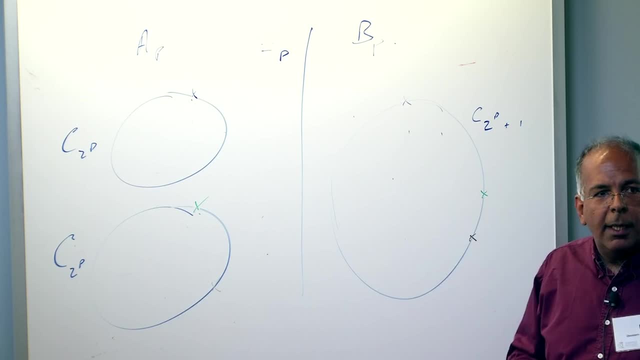 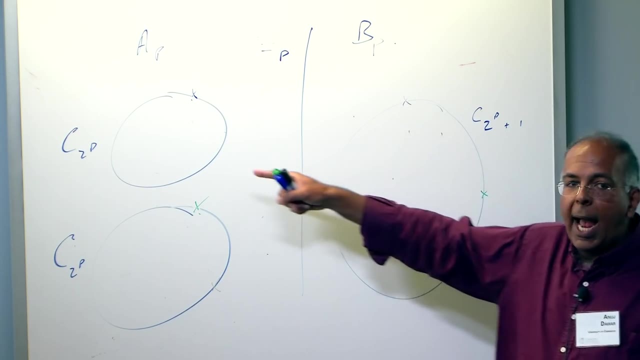 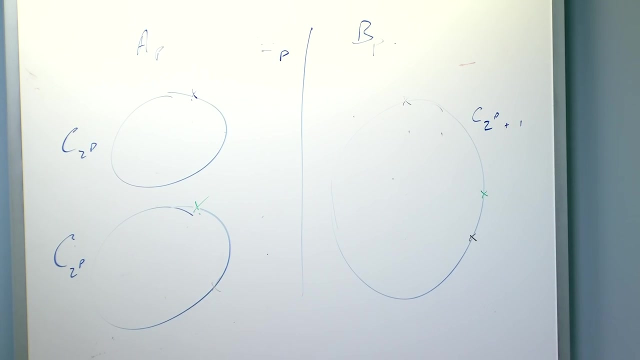 the number of moves remaining, And the idea is that the best that spoiler can do to force a win is pick something in the middle to cut the distance in half, and duplicate can survive p rounds of that. That's the essential idea. So these two things are p equivalent. 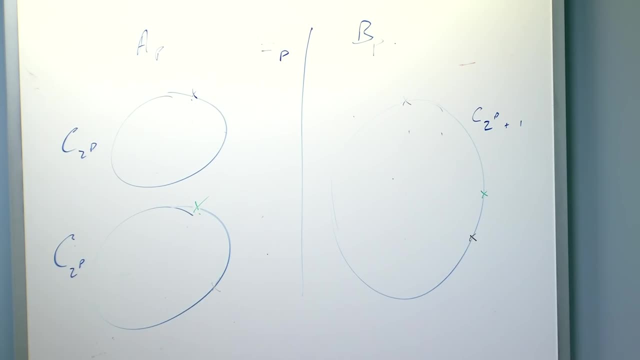 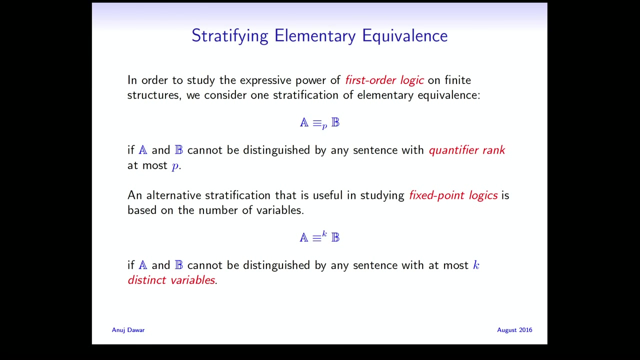 and, as I said, the undefinability of all of those properties follows An alternative stratification we will consider which is useful in the study of fixed-point logics. I'm not going to get to fixed-point logics until later, but I thought I'd mention. 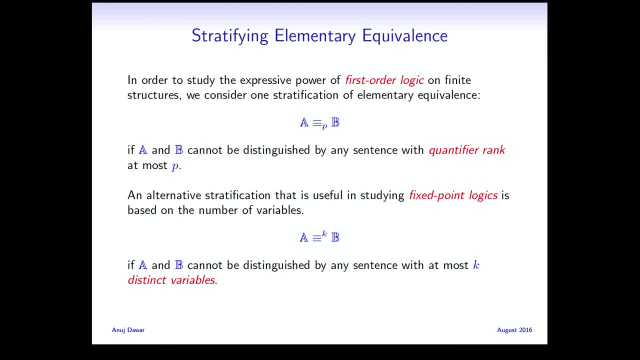 this at this point is we say two structures, A and B, are indistinguishable, and now I'm using superscript k to mean that they can't be distinguished by any sentence which uses at most close to the same number of moves remaining. So if you have a structure A and 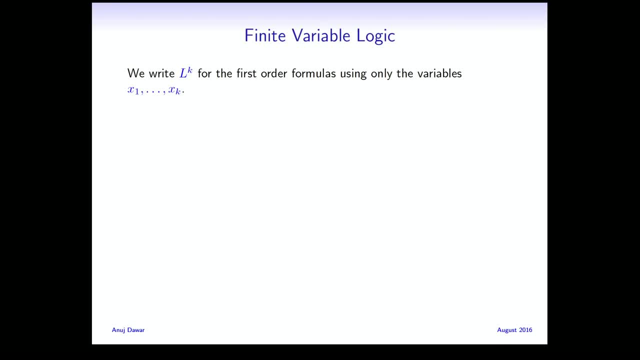 B, you have a set of k distinct variables. This is a very different measure. Let me sort of define it very quickly. So we write Lk for the first order formulas which use only the variables x1 through xk. So we fix a set of k variables and those are the only. 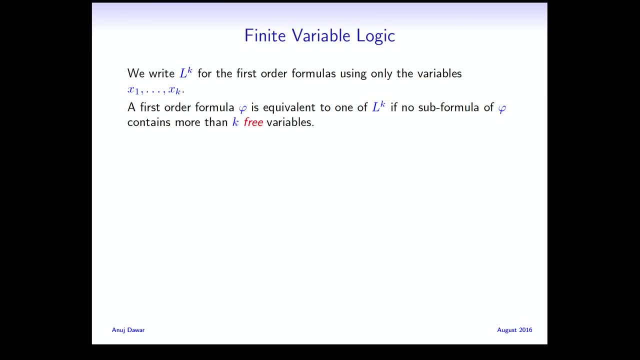 ones we are allowed to use in constructing the formula. Another way of thinking of this is this: is those formulas of first order logic in which no subformula contains more than k free variables. Because if this is true, you can just rename the variables to use just x1 to xk. But by simple renaming you will get a formula of: 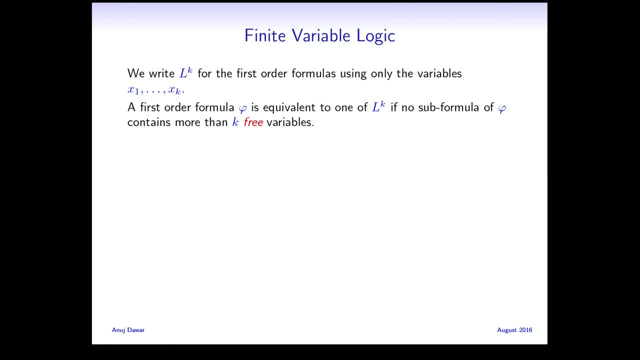 Lk. So this is a measure of the width of a formula. It's essentially. you can't refer simultaneously to more than k things inside your formula. Now, if two things can't be distinguished by any formula of at most k variables, they can't. 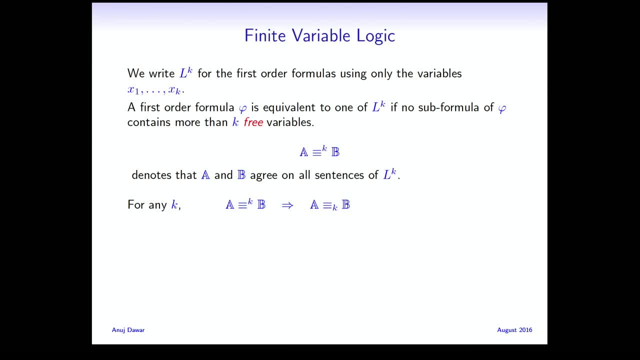 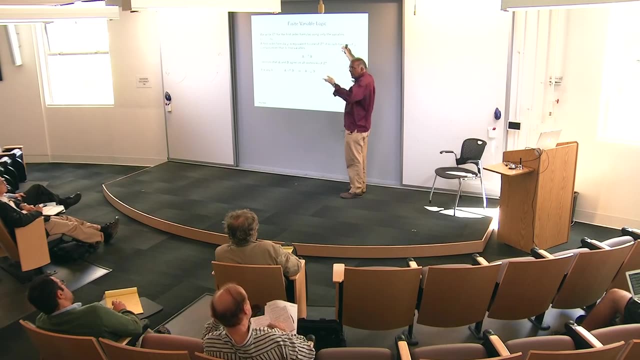 distinguished by any formula of quantifier rank at most k. Because any formula of quantifier rank, any sentence, I should say of quantifier rank at most k again, can be rewritten to use at most k variables, Because clearly, if it's a sentence has no free variables and 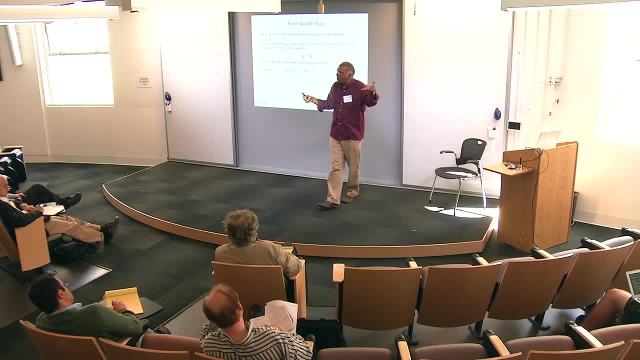 the quantifier rank is at most k. any subformula appears in the scope of at most k quantifiers, so it has at most k free variables. renaming variables, you get something in lk. The converse is clearly false, In fact in a very strong sense, for any p we can find. 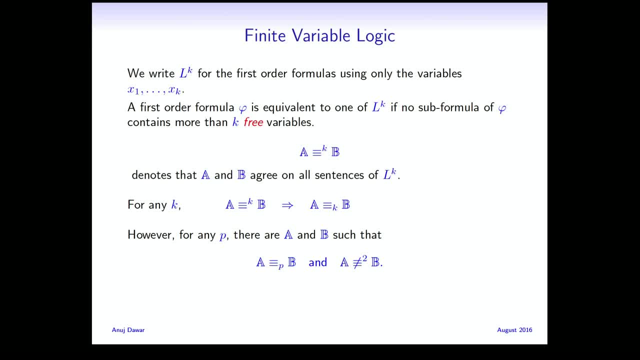 two things that are p equivalent but can be distinguished by a formula using just two variables. In fact, this example will do, or some version of that. You might have to make those graphs directed, but you can find a pair which are indistinguishable in quantifier. 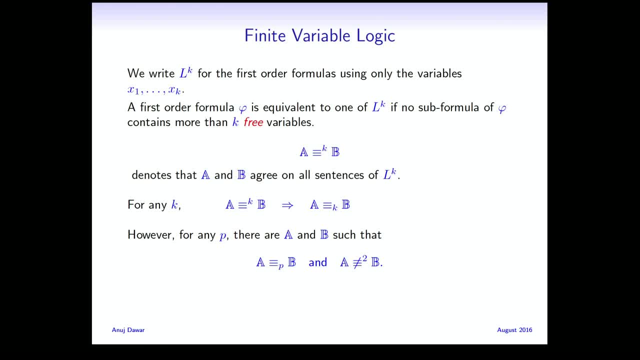 rank p, but distinguishable by a formula using just two variables, but high quantifier rank. You have to reuse the variables. So let me give you an example. So in particular, connectivity and two-colorability, even for undirected graphs, are axiomatizable in lk. But having an even number of elements is not. 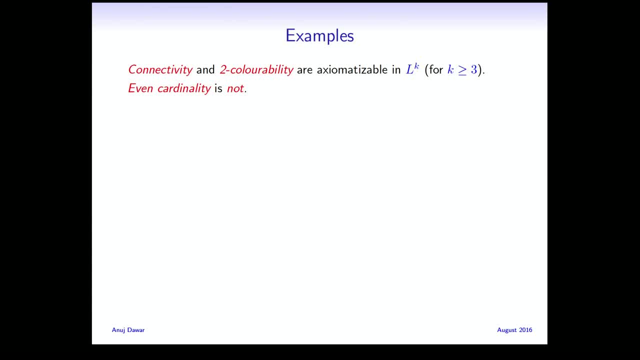 So of those three examples which I said, this one showed you first: order law you can't define. once we look at distinguishability in k variables, we get a difference between them. So let me see I've written down. I tried to write down a definition in for expository. 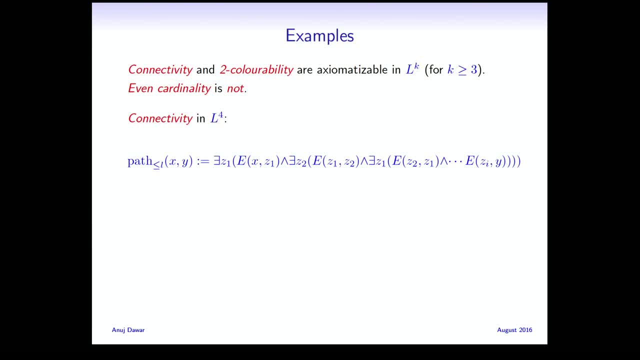 purposes, I've used four variables, but you can get away with fewer. a definition of connectivity, So here's one For every l. we can write down a sentence- sorry, a formula- with two free variables, x and y, using only two additional variables, which says that there's a path. 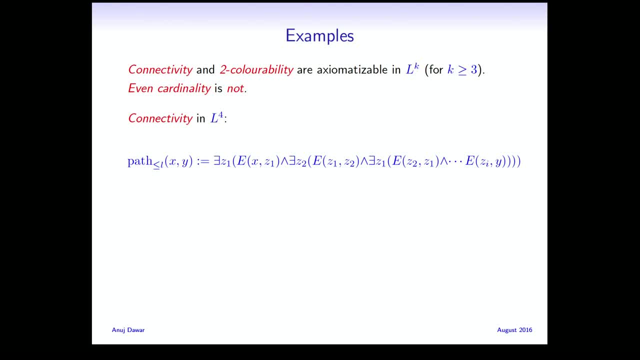 from x to y of length less than or equal to l. Now, l is arbitrary, but we're only using two additional variables. What do we say? We say there is an element z1, and there's an x from edge from x to z1, and a z2 with an edge from z1 to z2.. And we're going to 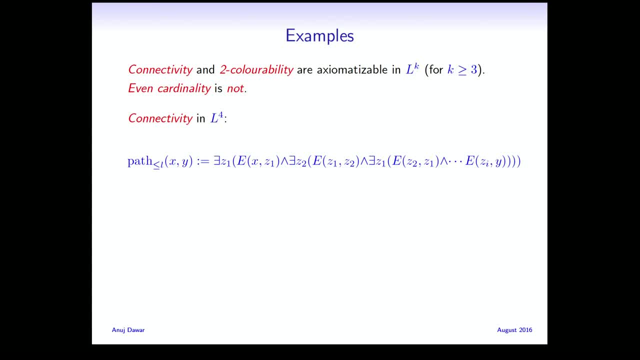 go on like this to say there's a sequence of l elements which takes us to y. But the point is that once we've said there's a z2,, we can reuse the variable z1, because we don't need it anymore. Say there's a, so x has a successor, z1, which has a successor, z2, which has a successor. 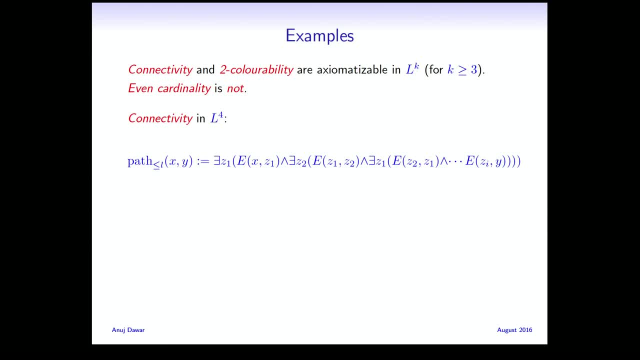 z1,, which has a successor, z2,, et cetera. And then we're going to say, well, we've got a step, And in l steps we then say we get to y. That should be l minus 1, I suppose. 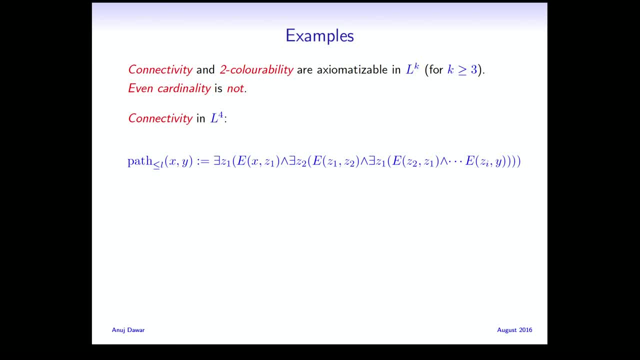 rather than i. But right in l steps we get to y. We've used a total of four variables for our arbitrary l. Now I write a sentence which I've called disconnect l, which says the following: For every x and y, if there is a path from x to y of length at most l, 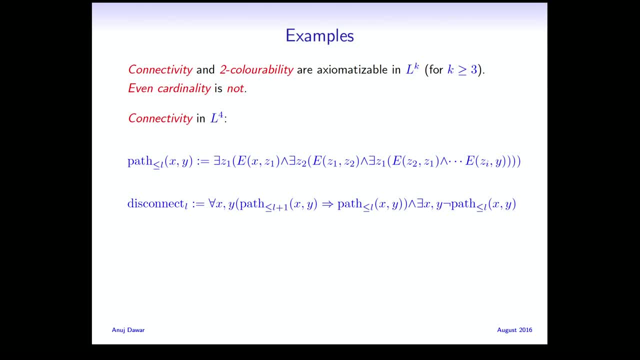 plus 1, there is one of length, at most l. OK, so there's no path, no things in the graph with distance greater than l, But there is a- sorry that r- where there is a path. but if there is a path, effectively what this says is, if there is a path, there is one of. 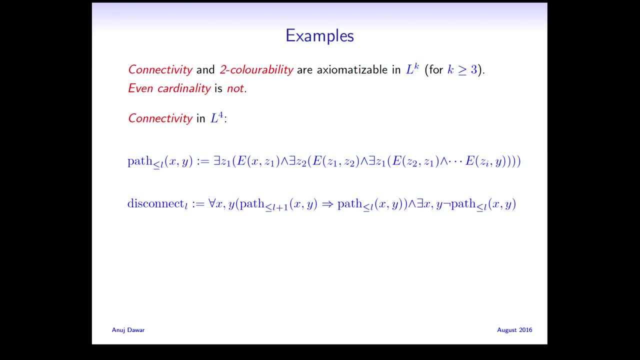 length at most l, But there is a pair of points for which there's no path of length l, Right, so this describes graphs which are disconnected but in which every pair of points in the same connected component have distance at most l. And now this infinite collection of sentences. 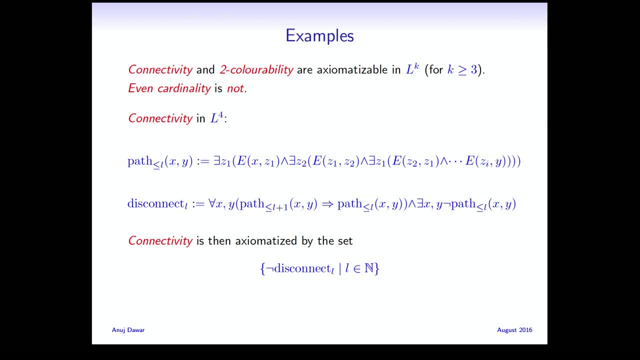 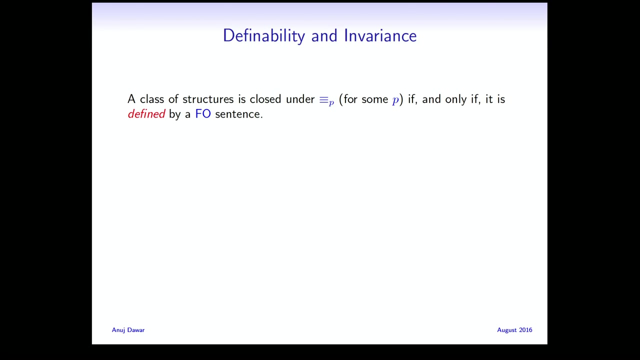 which is the negation of these for all l. L defines the connected graphs. The graphs which satisfy this for all values of l are exactly the connected graphs, And this is a theory using, as I've written it, no more than four variables. OK, but you can't do it in first order logic, OK, so I've already. 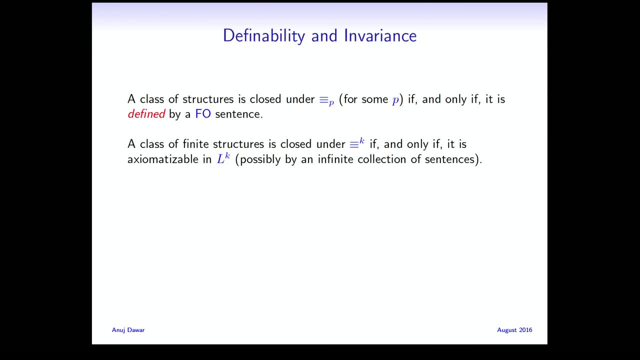 said, this Class of structures is closed under p equivalents for some p if, and only if, it's defined by first order sentence. It's closed under k equivalents if, and only if, it's axiomatizable in l, possibly by an infinite collection of sentences. OK, 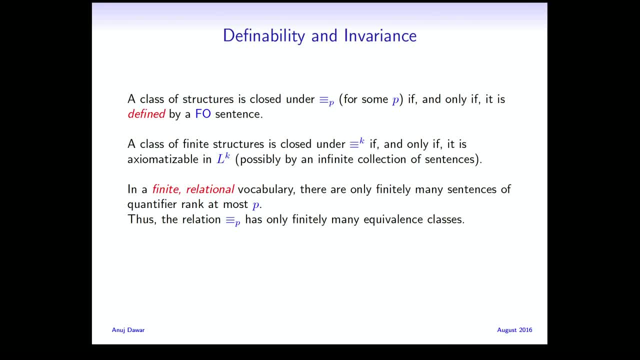 Because there are only finitely many sentences of quantifier rank, at most p. this equivalence relation only has finitely many equivalence classes, But on the other hand the k variable equivalence classes already for k equals 2 and any larger values has infinitely many. 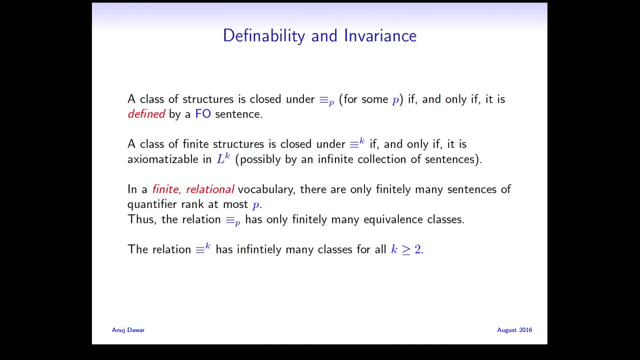 equivalence classes. OK, I mean, yeah, this is not very hard to construct the examples. I mean, I say I made the claim for k greater than 2, but you can take the connected graphs- example I had on the previous one- and certainly for k equals 4, that already gives you examples of this. So this k-variable. 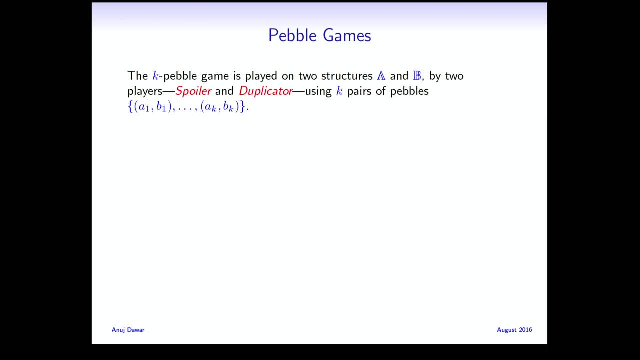 equivalence relation has a similar game characterization. We call this the k-pubble game. Again, it's played by our friends Spoiler and Duplicator, playing on a pair of structures, A and B, And the idea is the following. now, This is to capture the idea that in this k-variable logic, essentially 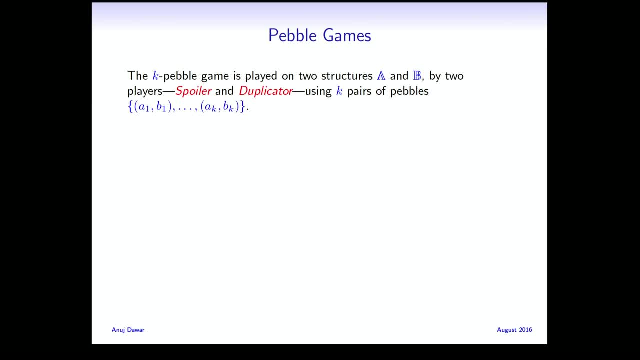 you have to reuse variables to say something meaningful. So, as before, Spoiler and Duplicator pick elements of the structure, but they have limited resources. They have k positions they can point to at any given time And after that you can carry on the game beyond k moves. 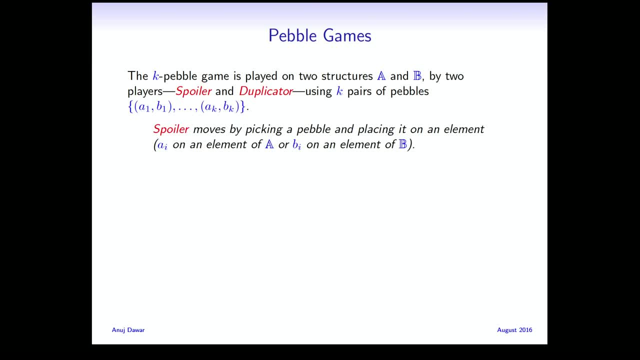 but you have to move the pointers, So we call them pebbles. So at each move, Spoiler moves by picking a pebble and placing it on an element of one of the structures: an element of A if it's one of the AIs, an element of B if it's one of the BIs. Duplicator has to take 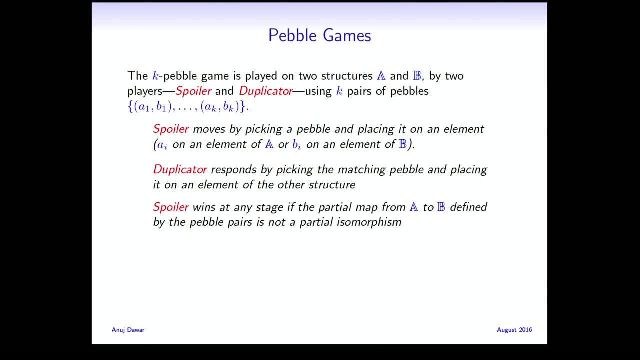 the corresponding matching pebble and put it in the other structure And again you look at the map defined by the pebbled elements. If it's not a partial isomorphism, Spoiler has demonstrated that these two structures are different and won. 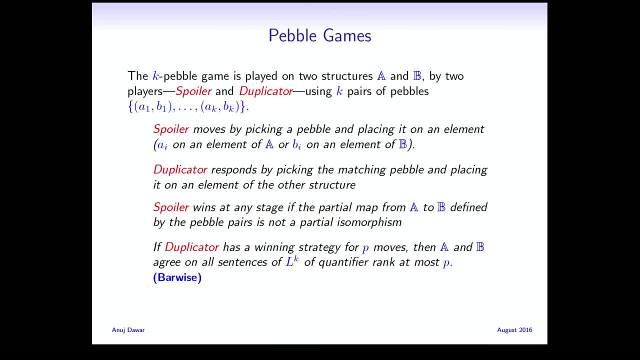 the game. And now you say: if Duplicator has a winning strategy for p moves, then the two structures agree on all sentences of Lk, of quantifier rank, at most p. And the key point is: p can be much bigger than k, in which case you will have moved pebbles from one place. 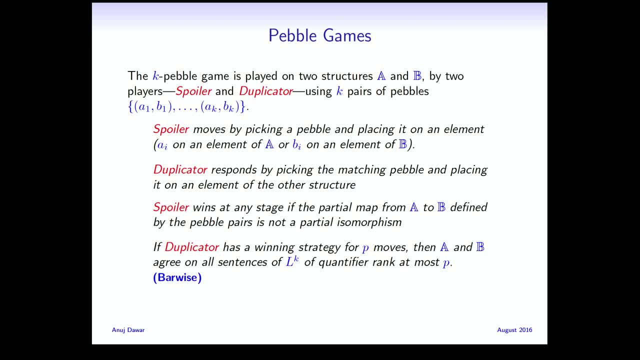 to another during the course of the game. The number of rounds you play for can be much bigger than the number of pebbles you use, And I mean- I'm not going to give a proof of this- It's essentially you, just you can. 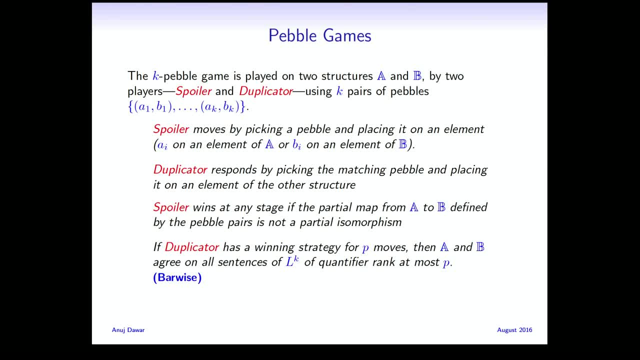 follow the lines, along the lines of what we had before. I'll just say this: I mean, what I've written over here is true for infinite structures as well as finite. But if A and B are finite, then there are only finitely many possible positions in the game. And if 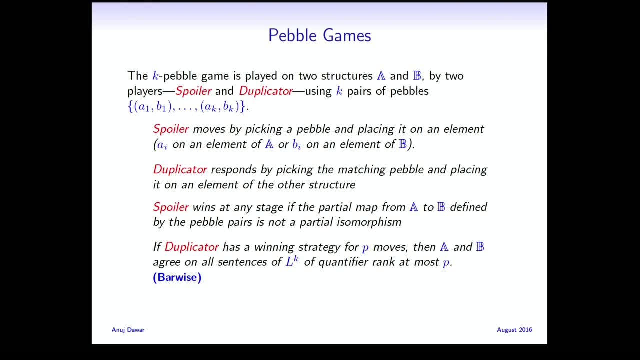 you pick p larger than the number of possible positions and Duplicator still has a winning strategy. that means Duplicator really has a winning strategy for playing forever without ever getting into a losing position. So two structures are k equivalent if, and only if, Duplicator has a winning strategy. 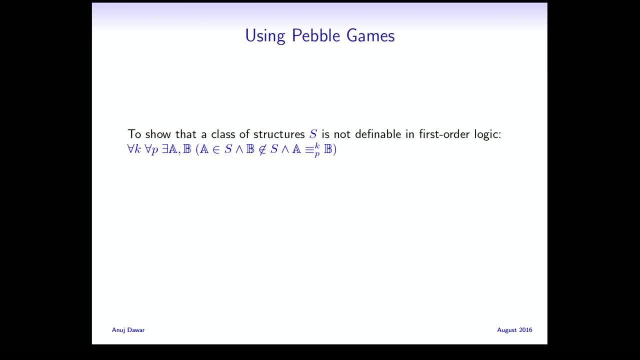 forever. This is specifically about finite structures now. So if you want to show that a class of structures is not definable in first order logic, what we typically do is, for every k and p, we find a pair of structures, One of which has a finite structure and the 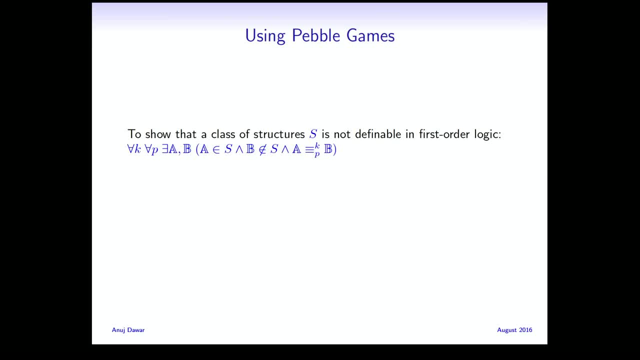 other is in the class and the other is not and they're equivalent. But because you can always bound the number of variables by the quantifier rank, we usually just forget about the k, And that's what we did before. If we want to show that something is not axiomatizable. 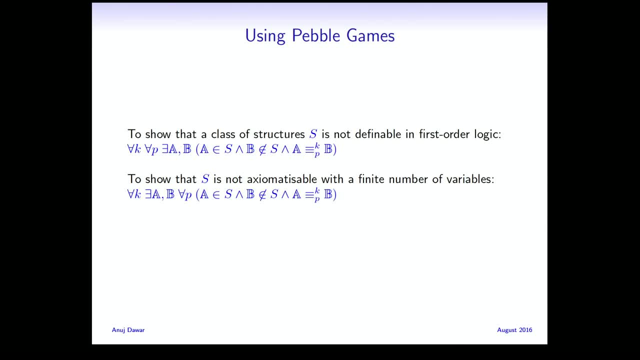 with a finite number of variables. what we need to show is: for every k, we can find a pair of structures, one of which has the property and the other doesn't, And they're equivalent for all values of p. kp equivalent, yes. 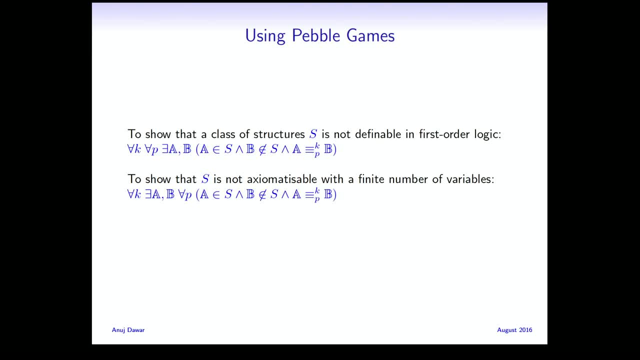 I'm still a bit confused. When you say not definable in first order logic, you mean not definable by a single set, By a first order set. yes. When you say axiomatizable with a finite number of variables, you mean 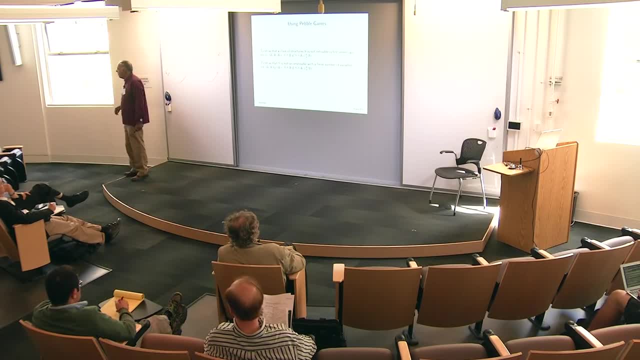 Axiomatizable by a theory. yes, By theory, Yes, right. So I didn't say this, but I used the word definable and axiomatizable slightly differently. in that sense, yes, So when we want to show that it's not axiomatizable. 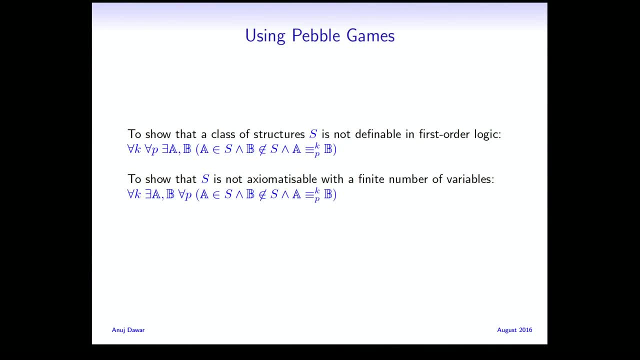 with a finite number of variables. this is what we typically show And here, as I said, because when the structures are finite, Proving it for all ps, it's enough to prove for p bigger than the size of, let's say, 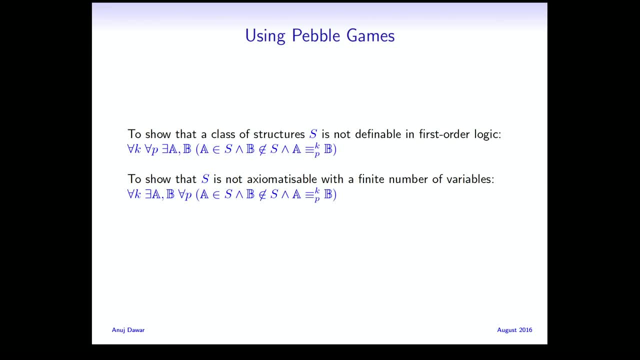 the structure raised to the power of k. we actually usually forget about the p and just say we're showing the duplicate. it can play forever. So here we can forget about the number of variables, Here we can forget about the quantifier rank. usually That's the way we. 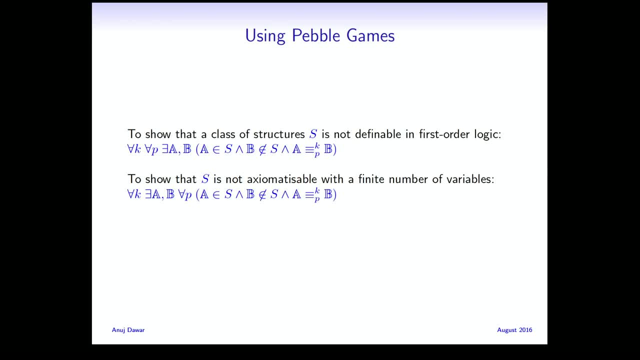 use these things. Something's gone wrong here. as you can see, Evenness is not axiomatizable with a finite number of variables, because for every k there are structures where a k has an even number of right. So I showed you this example to show you that connectivity, two-colorability and evenness 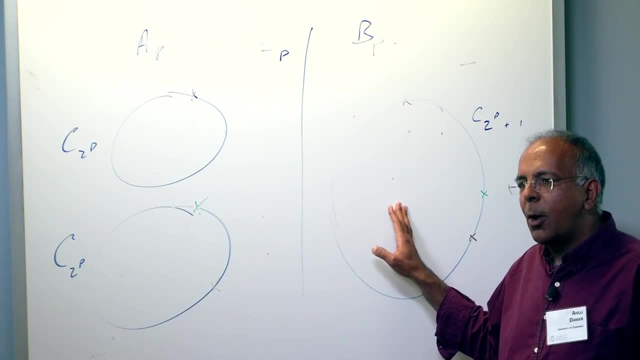 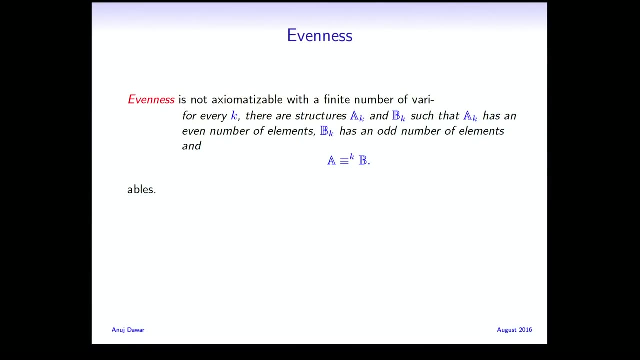 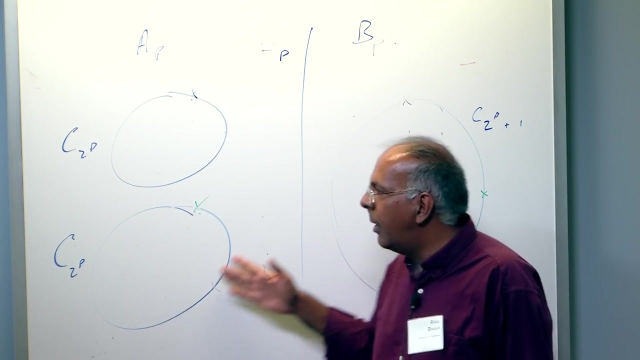 with a single example are not first-order definable. and I said connectivity and two-colorability are axiomatizable with a finite number of variables, but evenness still isn't. And this is actually very simple. you just take any structure with k elements here and 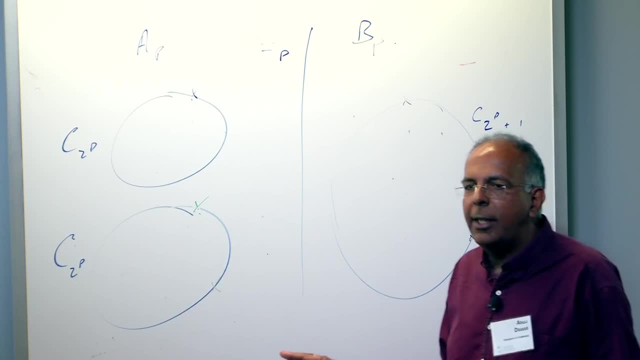 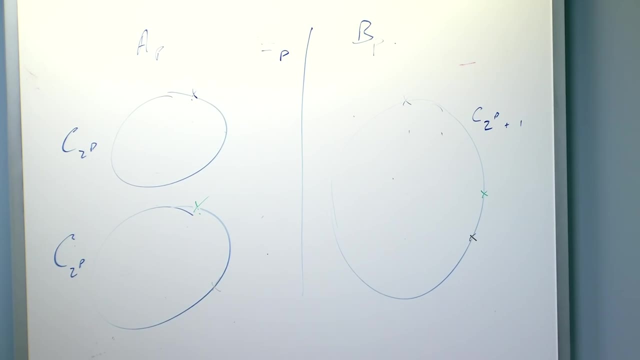 a structure with k plus one elements here, no relations on them whatsoever. okay, And the only relation is equality. and you see that Duplicator has a strategy for playing forever Because you match any move of spoiler on one side. Okay, 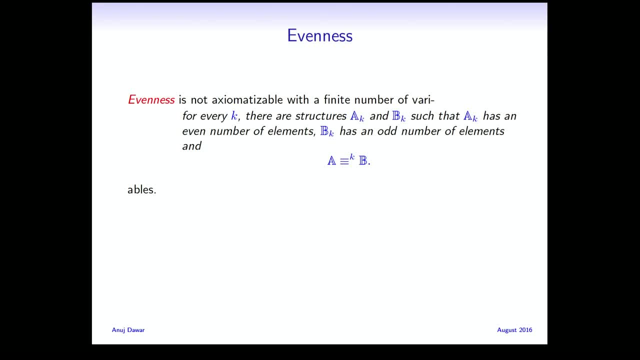 By picking an element. that's well. if spoiler plays on an element that's already pebbled, you play on the corresponding element. on the other side, Spoiler plays on an element that's not currently pebbled, because there are, at most, k pebbles. 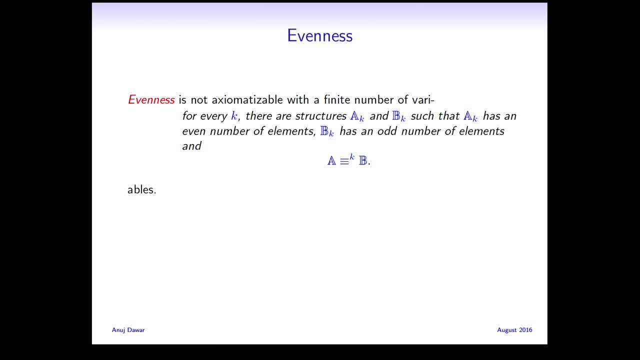 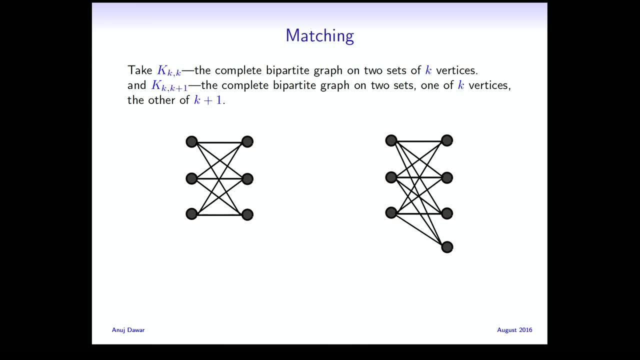 there is at least one on the other side that's not pebbled, and you place it there and all equalities are always satisfied. So Duplicator can just carry on forever. okay, Here's another example to make this a little bit more interesting. 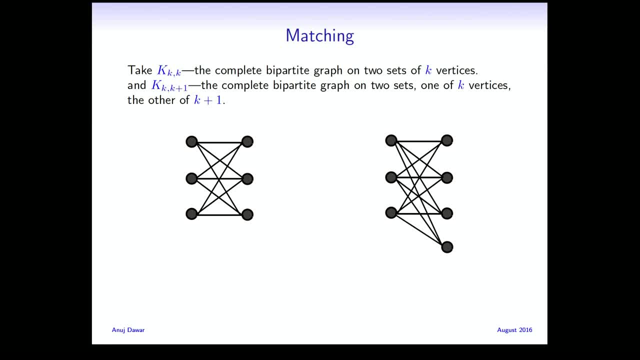 Take the complete bipartite graph on two sets of k elements. and this is the complete bipartite graph with k elements and k plus one elements. okay, for the special case, k equals three And the claim is now again. you play the k pebble game on this and Duplicator has. 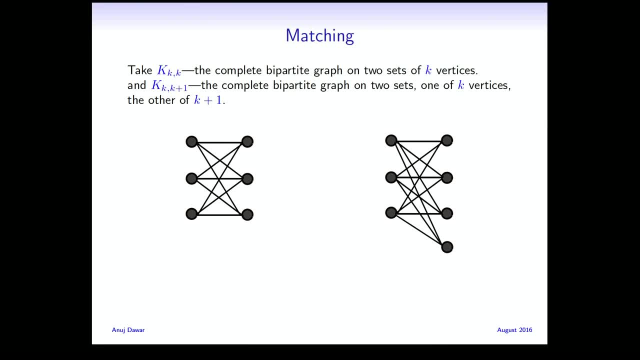 a strategy for playing forever, because you match any move of spoiler in this part with a move on this part and vice versa, any move on this part with a move on this part, and vice versa. Because there are more than k in each part, equalities will always be satisfied. 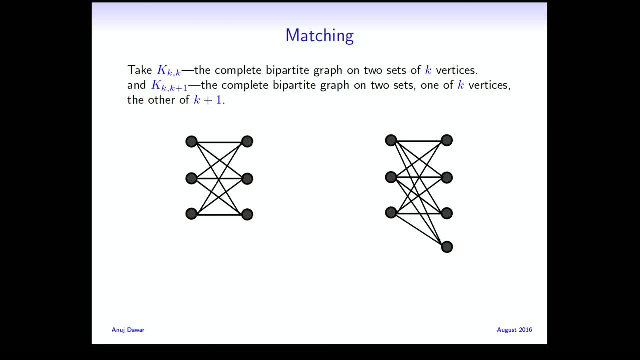 You can always find an element not equal or equal to the others as necessary, And between the parts there's always an edge, so that's also satisfied. So what can we say? These two things are equivalent, but this graph has a perfect matching, and this one 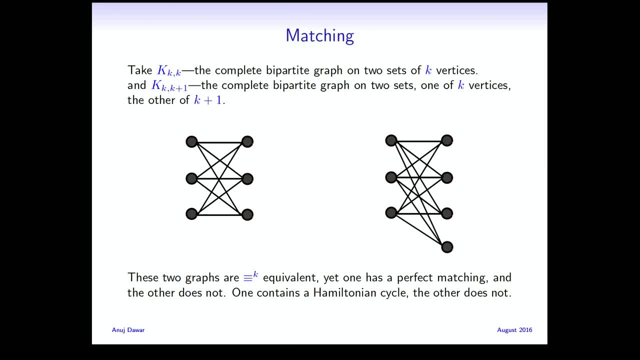 doesn't. Therefore, the property of having a graph, having a perfect matching, is not axiomatizable with any finite number of variables. Also, turns out that this graph has a Hamiltonian cycle and this one doesn't right because you can, there's your Hamiltonian cycle. 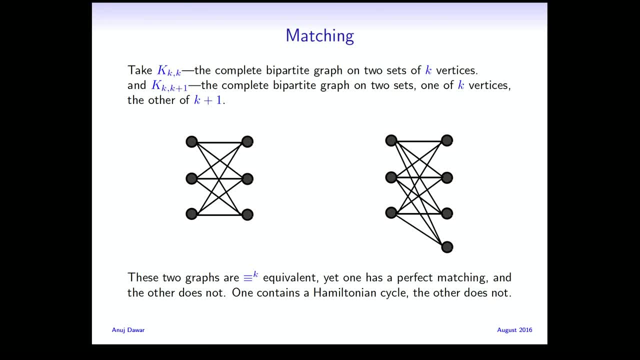 To see that this one doesn't notice that each stage of the cycle you have to cross from one part to the other, and since there's more elements on this side than that, you can't do that without repeating a vertex, right, if you're going to visit every one. 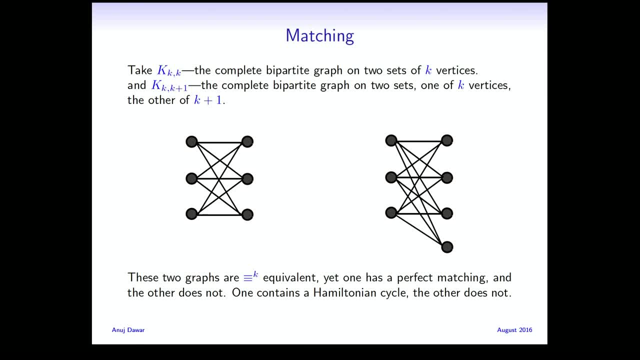 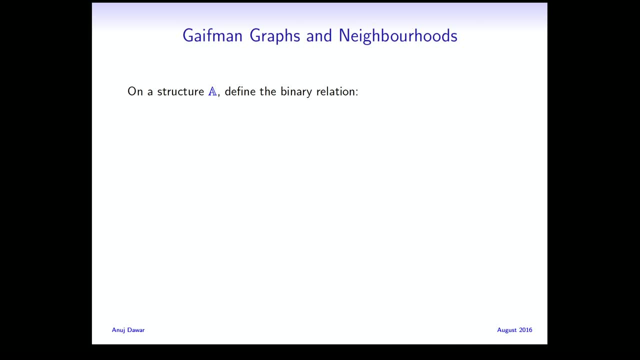 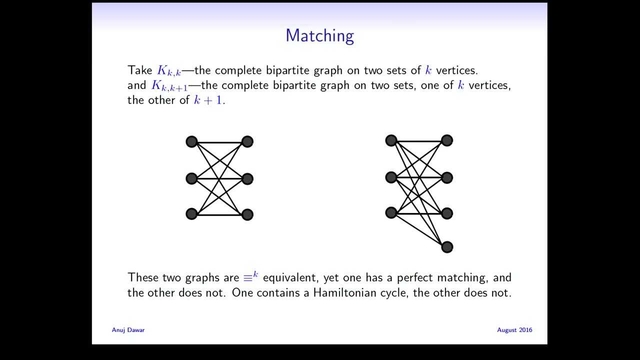 So the property of having a Hamiltonian cycle is not axiomatizable with a finite number of variables. Okay, Okay, Now let's see Finish at 12, right, So I'm going to come back to the uses of these finite variable logics later. 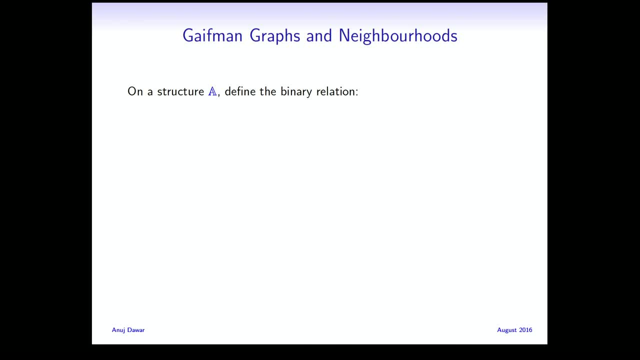 I just wanted to say a little bit about, as I said, I wanted to get to talking about locality, and this will be the last thing I'll say. To define what I mean by locality. it's useful to define, given a structure, A look at the. 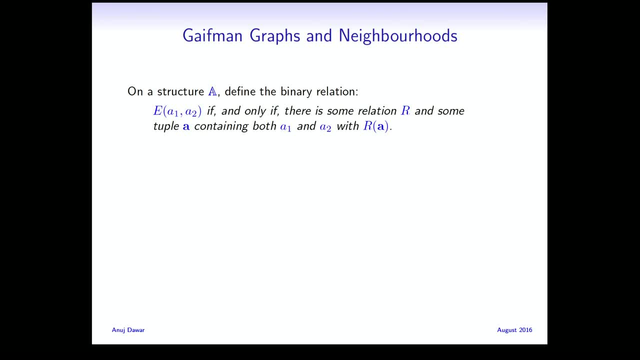 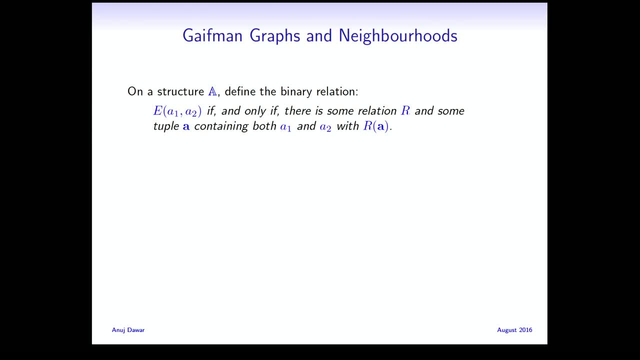 both elements Okay. So basically two things are related somehow by this structure. We call this the Graf of A. right, You take the universe of A along with this edge relation, which is a symmetric edge relation, so it's an undirected graph. 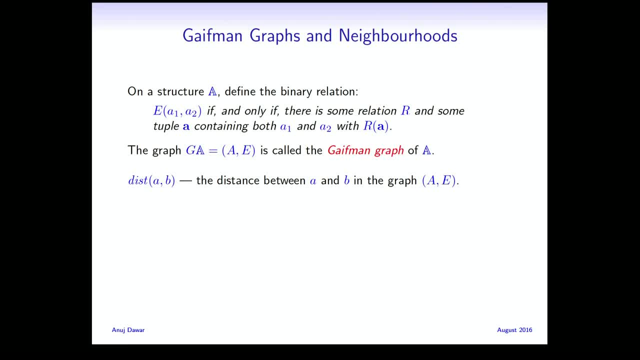 graph. And when I say, when I talk of the distance between two points in the structure, I mean the distance in this graph, the graph-theoretic distance, And I will talk of the neighborhood of an element A. This means you take all the 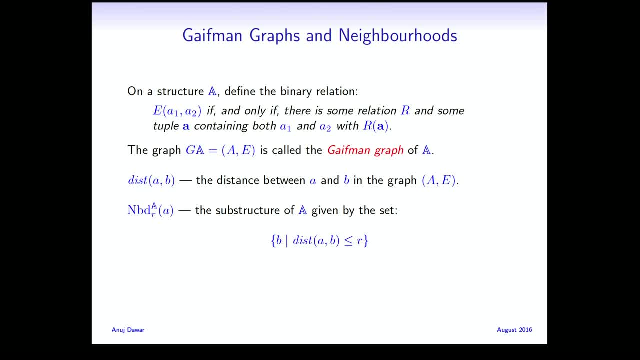 elements neighborhood up to a radius r for positive integer r, you take all the elements at distance, at most r to A, and you look at the substructure they induce. Okay, so this is a structure in the vocabulary of A. Okay, I call this the. 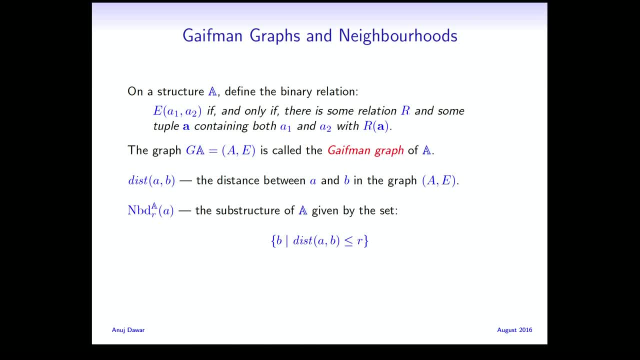 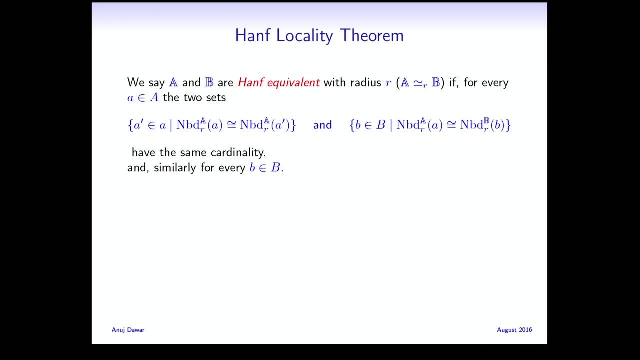 r-neighborhood of a single element. This allows me to formulate my first version of the Hanf locality theorem, which is the following: We say two structures are Hanf equivalent with a radius. If the following is true, I mean realize this is maybe not the most clearest. 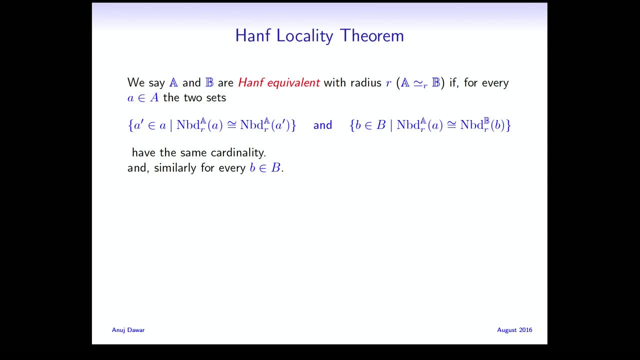 formulation of this, but I put it in this form because I'm going to introduce thresholds later and it's easier to do it this way. Let me give you the clearer formulation. Two things are Hanf equivalent with radius r If there's a? 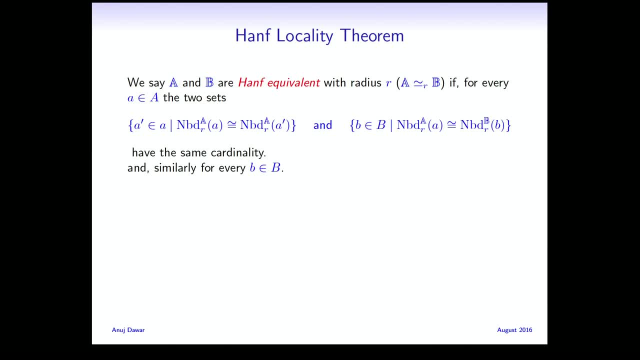 bijection between the two universes, between the two structures, so that for each element, its r-neighborhood is isomorphic to the r-neighborhood of its image. What I've written here is: there are an equivalent if you count the number. 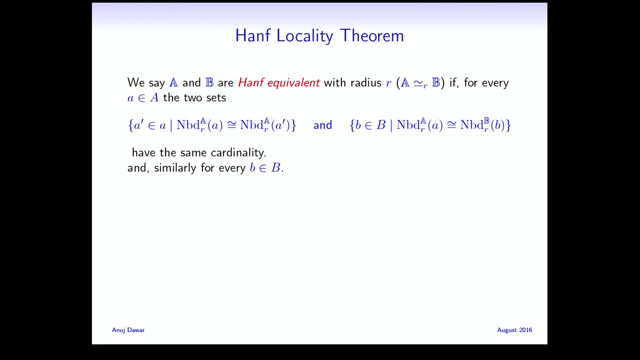 of isomorphic neighborhoods for each element and you count the number of elements which have isomorphic neighborhoods to A. in B they have the same cardinality, So you can put a bijection between them, And it's the same for B. So for each element of B you count the number of neighborhoods in A. 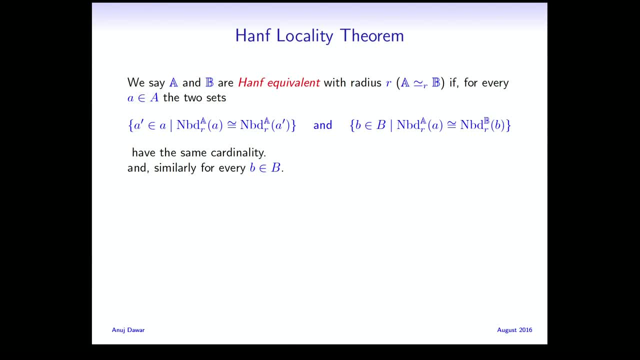 which have the same, which are isomorphic, and you count the number of neighborhoods in B which are isomorphic and they have the same number of elements. That should be a capital A there, Sorry, Which one At the beginning? A prime. 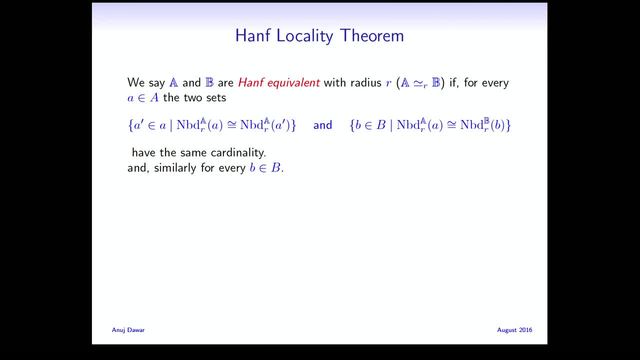 Yes, this one's a capital A. thank you, yes, Okay, and the Hanf locality theorem says: for any vocabulary and any p, you can find a radius r, at most 3 to the p. 3 to the p is enough, so that if you have a radius r, you can find a radius r at most 3 to the p. 3 to the p is enough, so that if you have a radius r at most 3 to the p, 3 to the p is enough, so that if 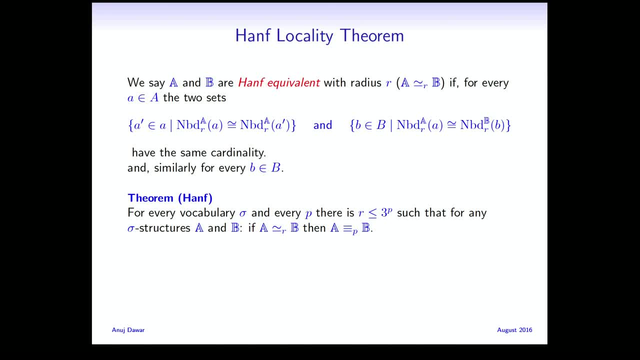 A and B are Hanf equivalent up to radius r, then they're not distinguishable in any first-order sentence of quantifier rank, at most p. So if the neighborhood's up to a fixed radius, the kind you look at, the multi-set of 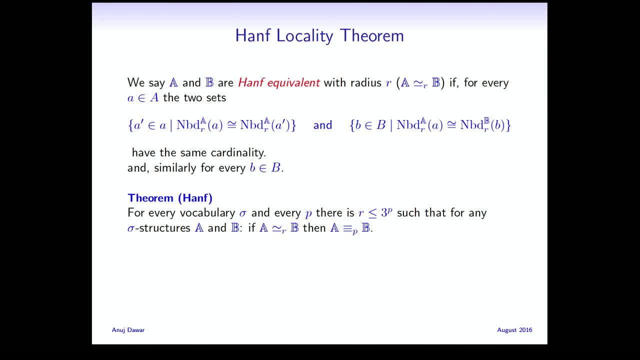 neighborhoods that appears in A and it is the same as the multi-set of neighborhoods that appear in B, then you can't distinguish them, Right? so first-order logic really talks about local neighborhoods. is what this is saying, Right? And I have a. 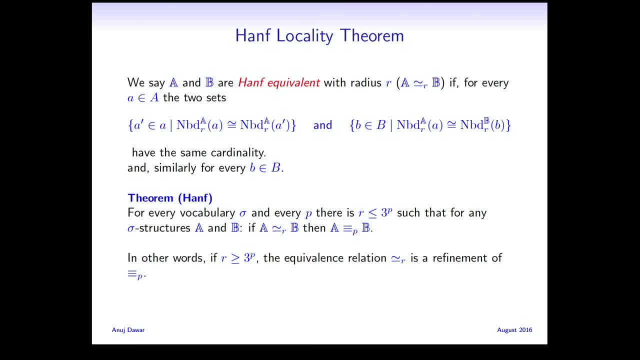 I have five minutes. I think I can sketch you a proof of this, and that'll be a good point to stop then. So what's the proof? The idea is, we want yeah, Just in this definition. how is it that it's an equivalence while the definition is not symmetric in A? 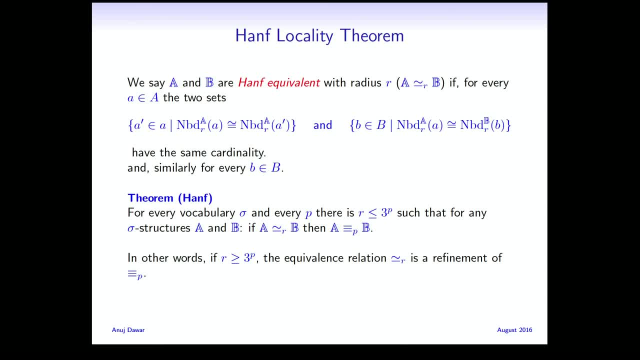 No. similarly, for every B means the symmetric bit, right, Okay. So, yes, this is not the best formulation, as I said. That's why I said it's the existence of a bijection, which is a bit clear, Okay. So let me. I want to give you the idea of proving this. The 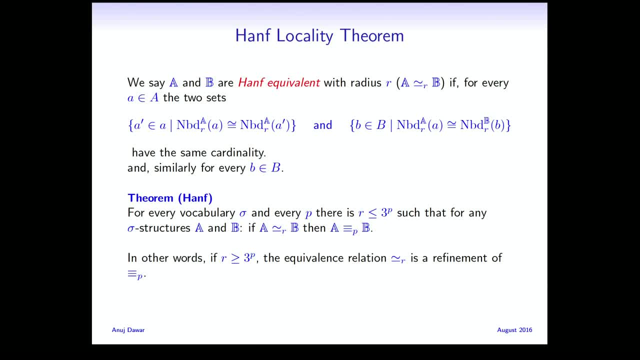 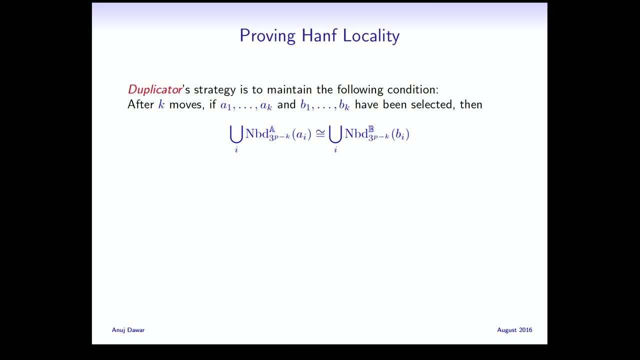 idea is, of course, we start from this assumption and we want to show that from that we can construct a winning strategy for duplicator in the p-round game. Duplicator strategy will be to maintain the following condition: So you have the structure, you have the 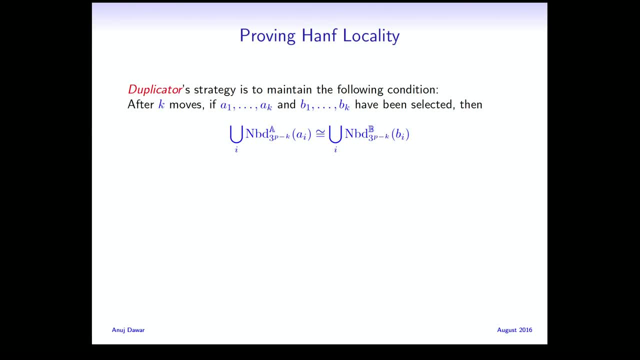 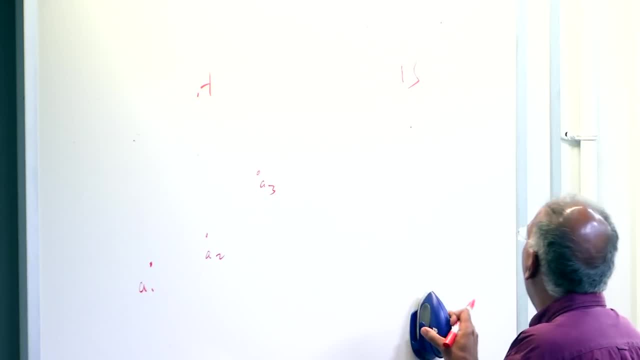 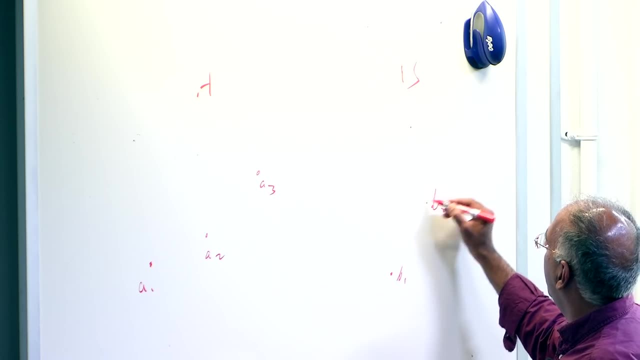 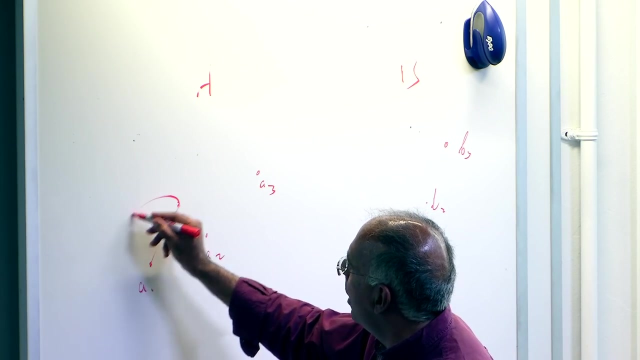 structure A and you have the structure B, and in here you have elements A1, A2, A3, right And over here you have elements B1, B2, B3, which have been selected in previous rounds, And what you do is you take the neighborhood. 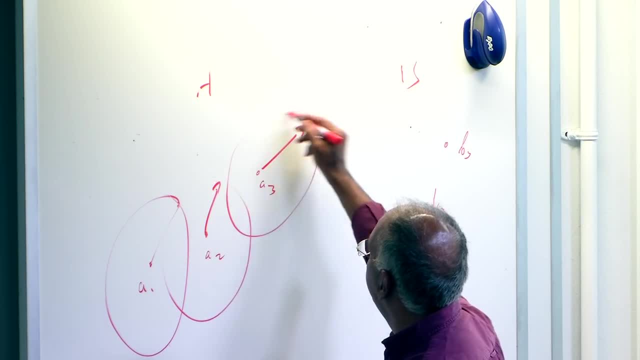 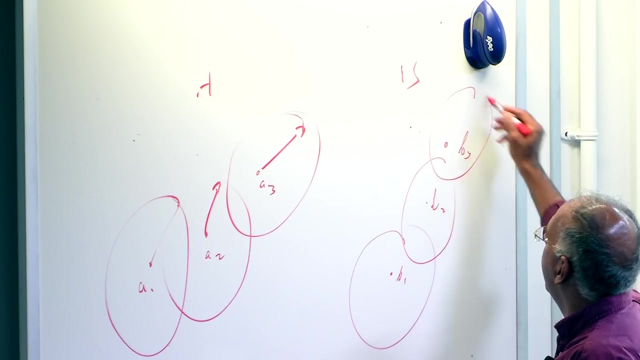 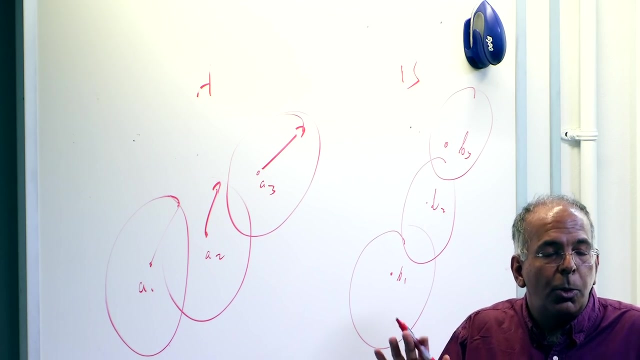 of B radius up to 3, raised to the power of the number of moves remaining to play around these points and you take the union of these neighborhoods And you have the same in B And duplicator strategy is to maintain an isomorphism between these two sets, between these two. 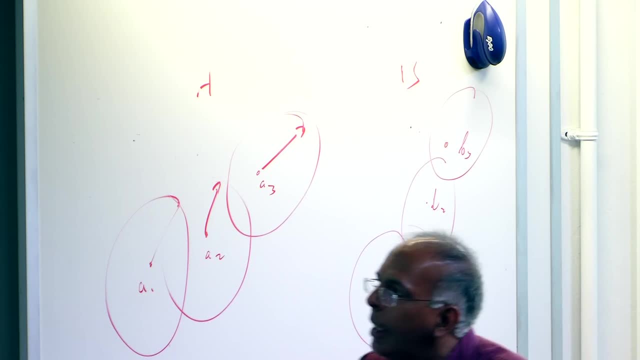 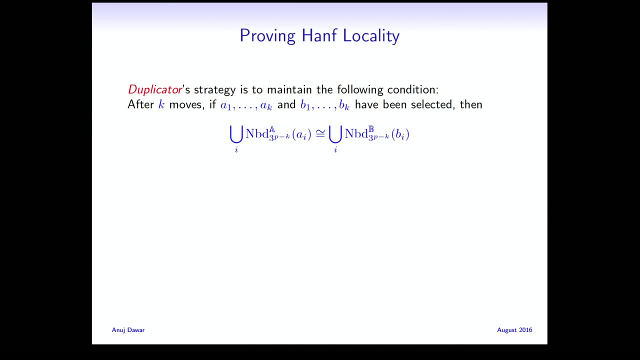 substructures. I should say, Okay, Why is this possible? Well, for the first move, it just follows from the, the definition. right, You pick one. you look at the neighborhood of radius 3 to the p. there must be one on the other side. 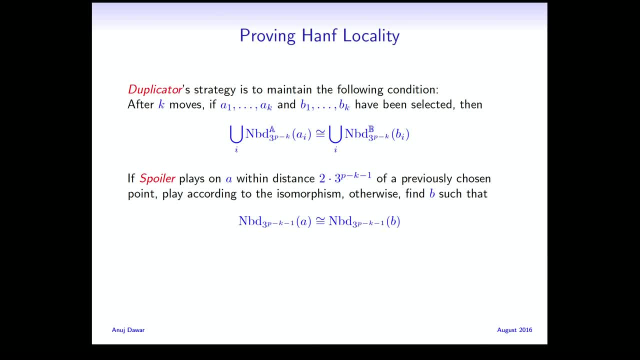 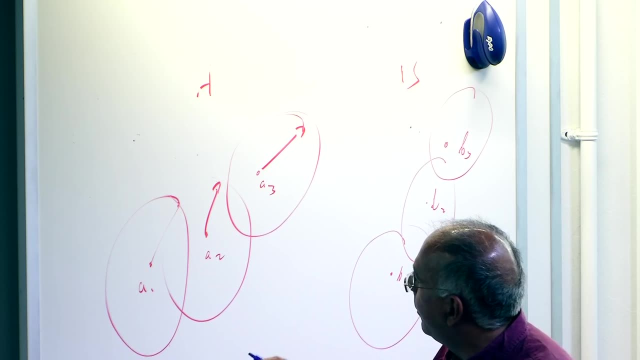 with an isomorphic neighborhood. Now we want to show inductively, this remains true. So suppose now spoiler picks an element, let's say somewhere in the structure, and we consider two cases, Either it is. so what are we going to do At the next move? we're going to shrink. 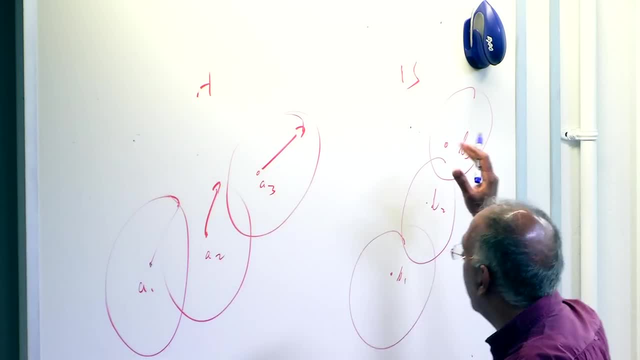 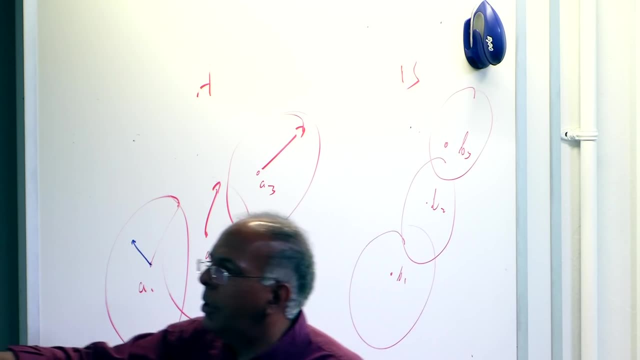 the radius of these neighborhoods. but we're adding one additional element and we want to do the same on the other side while keeping an isomorphism. Suppose this element that spoiler chooses is 2 times 3 raised to the power of the new right. 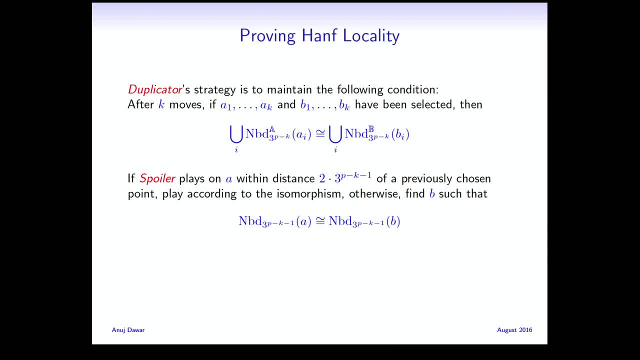 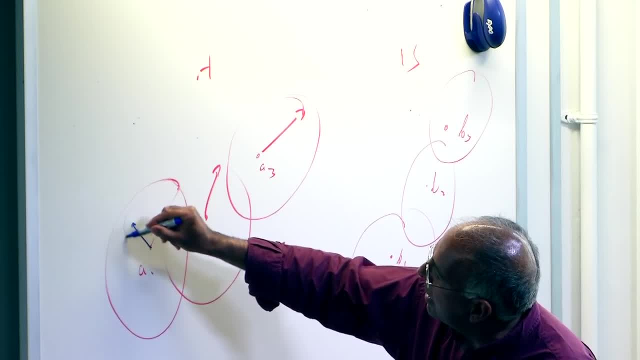 So 2 times 3 to the p minus k minus 1 means 2 thirds of this radius that I've drawn before. If it's within 2 thirds of that radius, that means its neighborhood of radius 3 to the p minus k minus 1. 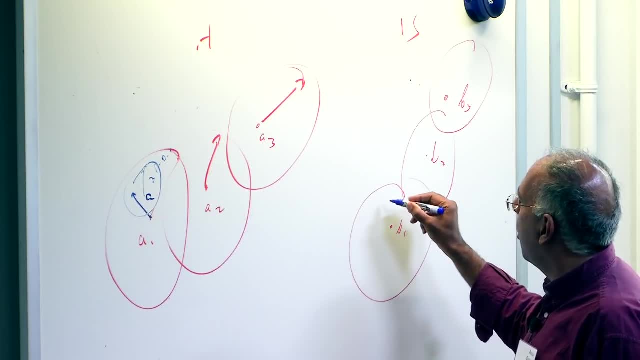 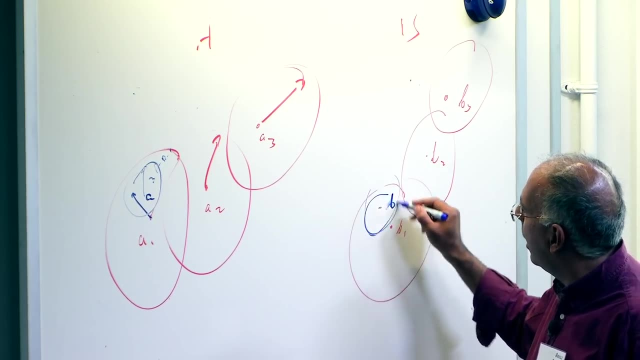 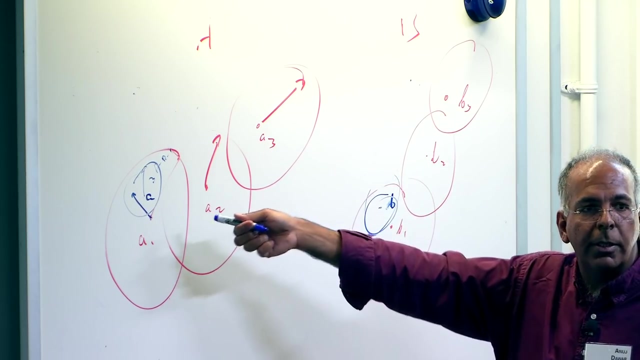 is entirely within this And therefore, by the isomorphism, there is an element here, b whose neighborhood? well, it'll be entirely within this, You know, because there's an isomorphism between these whole substructures, you pick the image under And you're done. 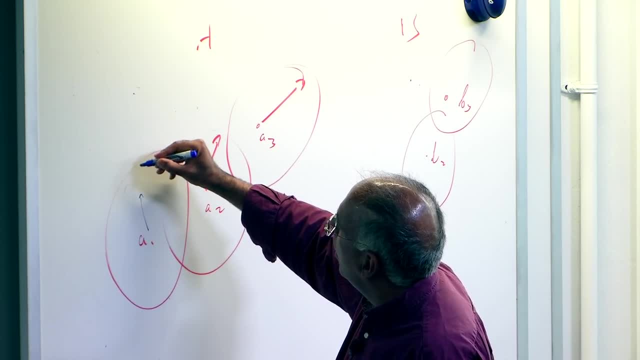 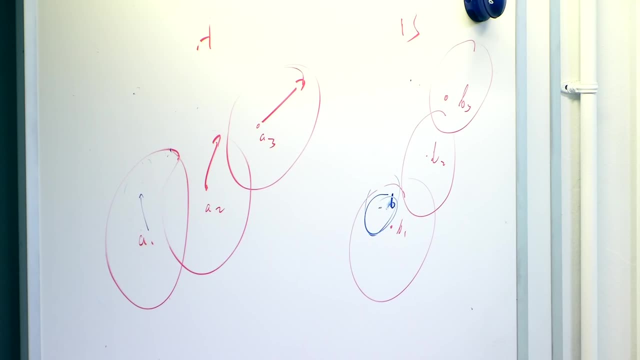 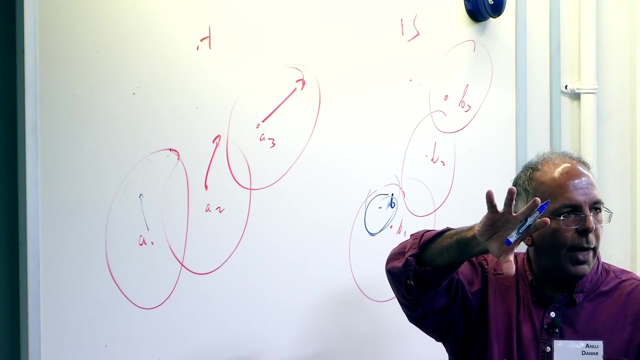 What happens if you pick an element here whose distance from any previously chosen element is bigger than that? Well, that means that when you shrink the size of the neighborhoods by a factor of 3, its neighborhood of radius 3 to the p minus k minus 1 will be disjoint. 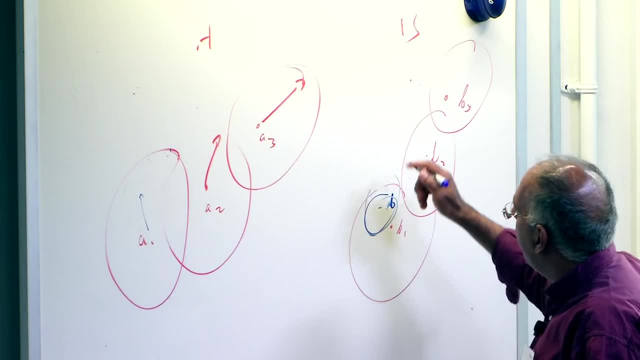 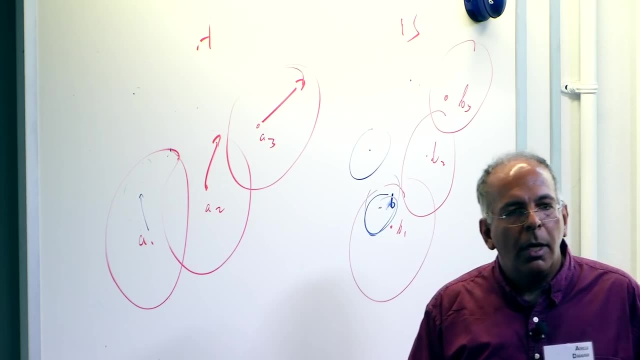 from all of these, And that means just by a count of the neighborhoods, there must exist a, b On the other side, whose neighborhood of radius 3 to the p minus k minus 1 looks exactly like the neighborhood of a And you pick that. 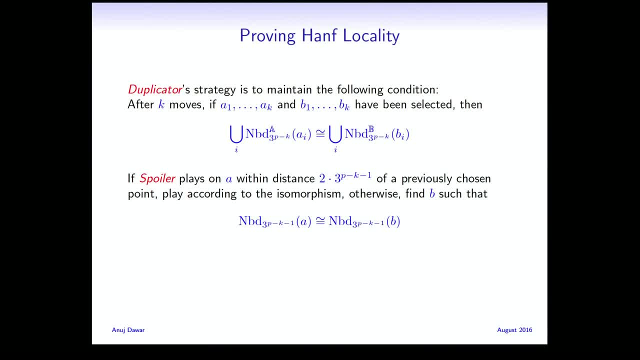 And it's disjoint from every, disjoint from this structure you had before. Okay, That's the essential idea. It kind of, if you look at it, it's a great generalization of this construction: Keep things far apart, things that are far apart. you can't. 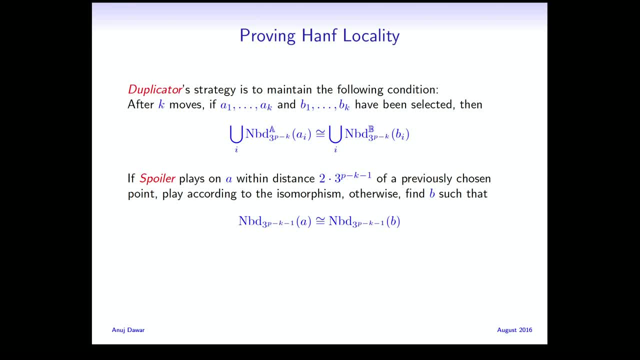 spoiler. it'll take a lot of moves for spoiler to show that they are actually different, And things that are close, you keep isomorphic. That's duplicator strategy, Okay, Okay, So that's, and we're going to look at certain applications of this and 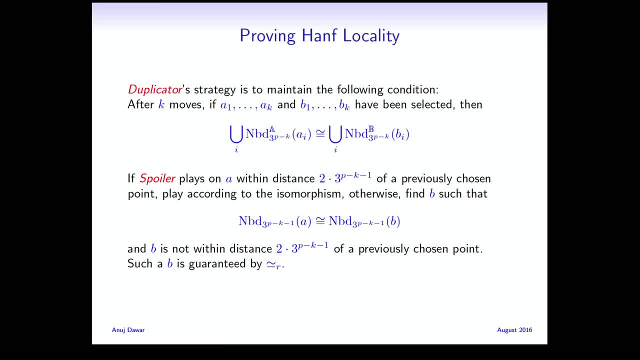 of the other locality theorem, Geismann locality, which I haven't got to, but I think I'll stop at this point And next time we'll look at some applications of locality and also automata theoretic methods. Okay, Applause, Applause. 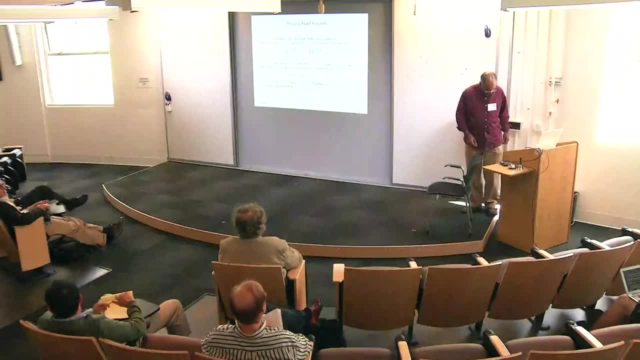 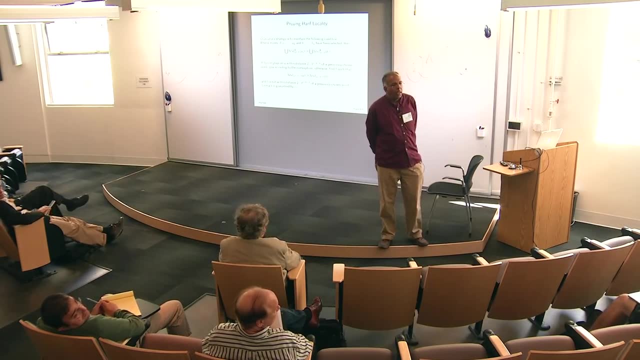 Applause Questions: Yes, But on your counting condition for Hock locality: you actually? Your statement on the previous screen was that the counts were equal. I think Yes, But actually all you need them is to be bigger than K, But then at a certain threshold. that's what, and I will. I will use that later. 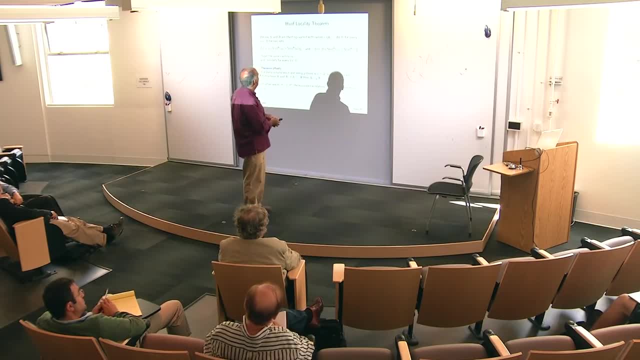 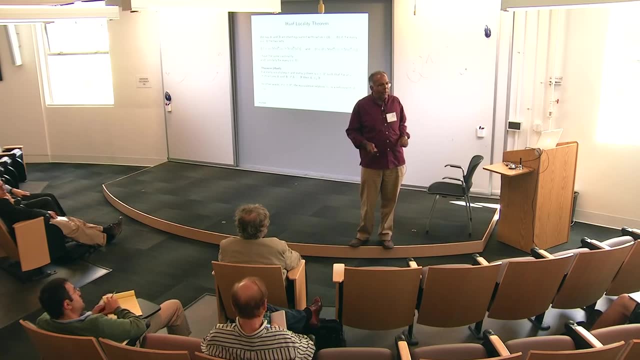 I mean I was going to. that's what I said. This looks unnatural. The natural way would be to say simply: there's a bijection between A and B, but I stated it in this form because later on I'm going to add a threshold to it doing exactly what. 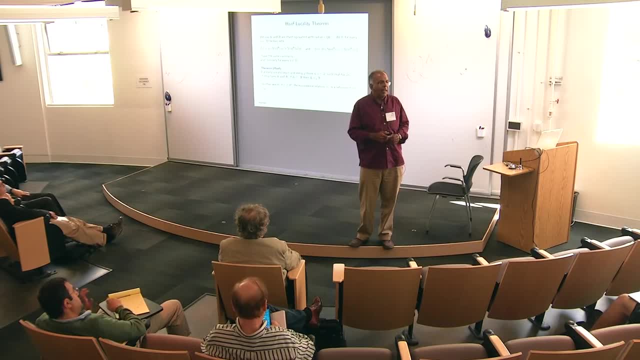 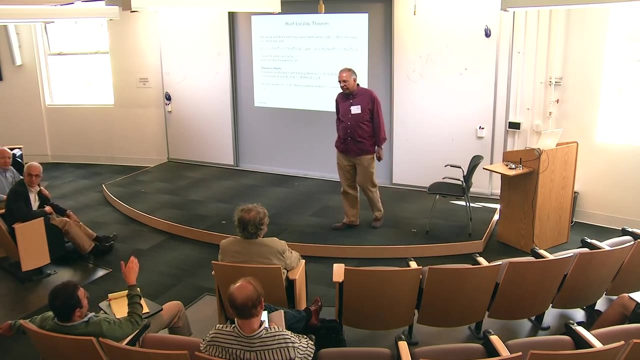 So you just say they have the same card and that way, or are both bigger than K, Exactly, exactly, Yeah, yeah, yeah, Okay, Any other questions? Okay, Kusho, Just kind of a comment rather than a question. is that you know, when we don't have locality?